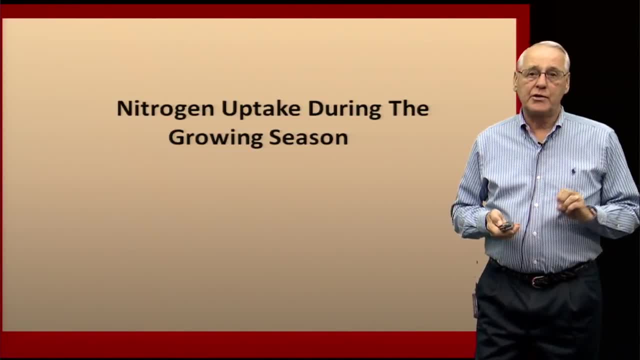 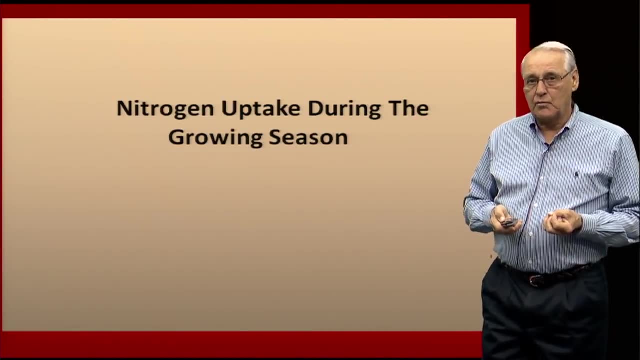 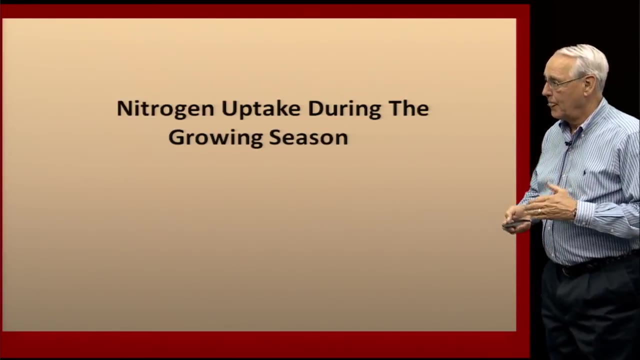 from the standpoint of nitrogen and water management to improve groundwater quality is that we don't want to over apply either nitrogen or water to lose nitrogen, and we have a number of management factors that can help us do that. So if we think about nitrogen uptake during the 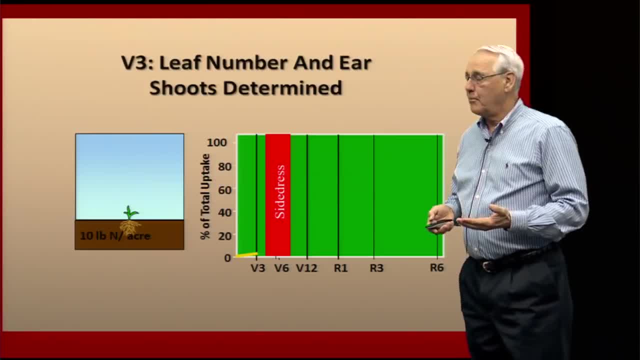 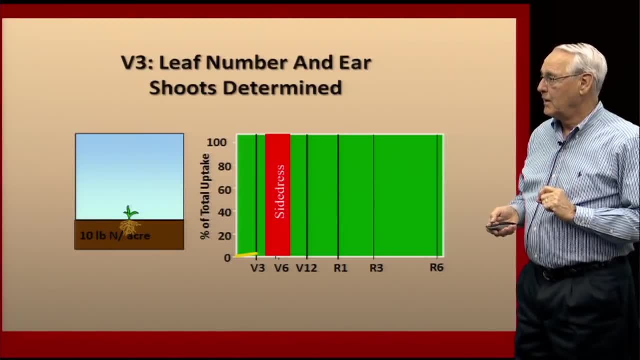 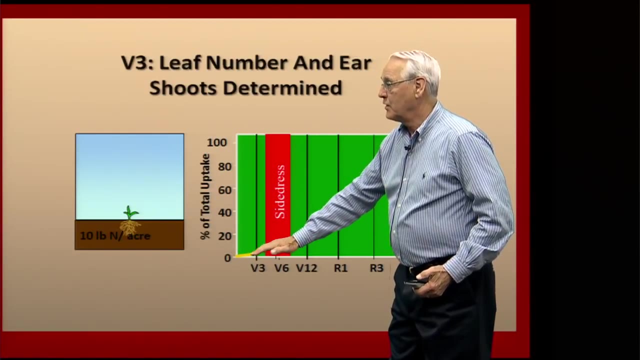 growing season. we've planted the crop, it's come up. we're at about the V3 stage, which means we have three true leaves. So at this point in the season, as you can see, we are taking up some nitrogen. but by this point in the season, as you can see, we're taking up some nitrogen. 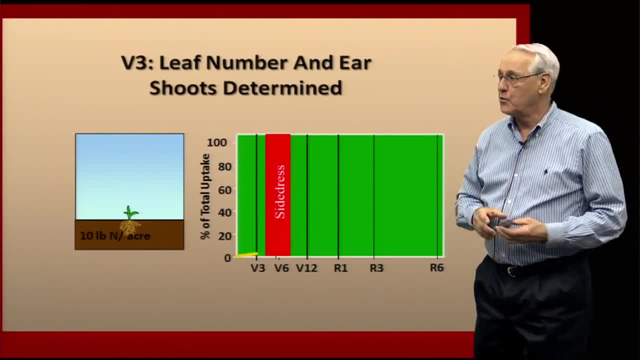 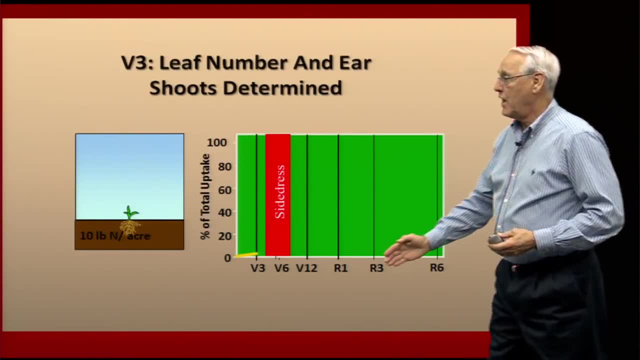 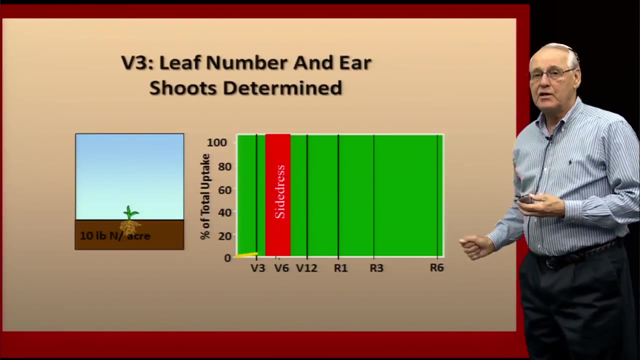 At this point in the season, at the three leaf, we've probably taken up only 10 pounds of nitrogen per acre. That's less than most farmers apply in a starter fertilizer band. So we're looking at going from planting all the way through R6, which is the vegetative stage of maturity. 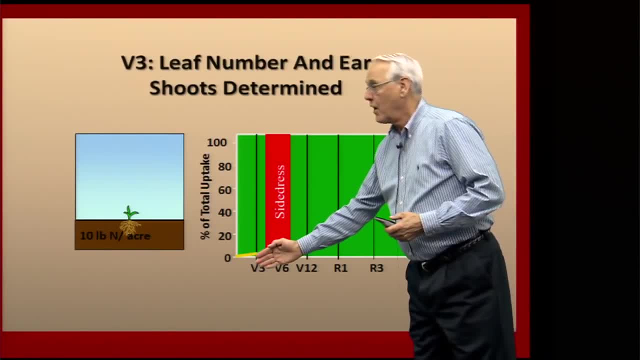 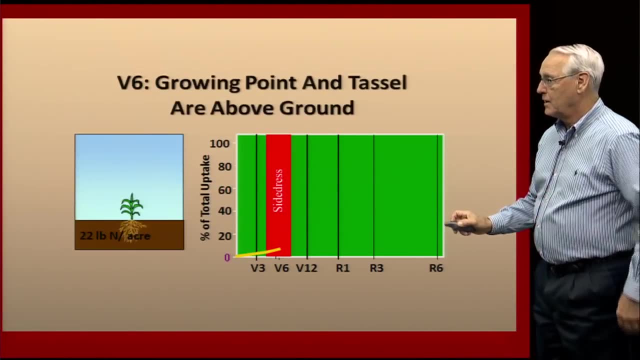 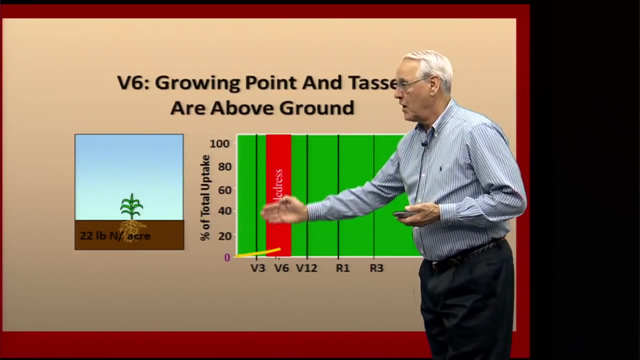 where the plant is matured. What we've noted on this graph is this kind of time window. in here we're thinking about side dressing nitrogen, So, as the plant continues to grow when we get to V6, we are really then into this time period when we think about what we call traditional side dressing. 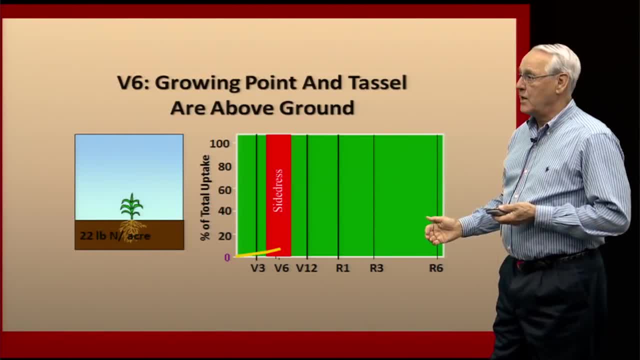 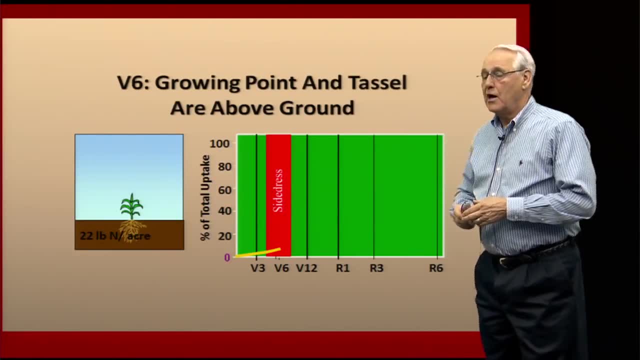 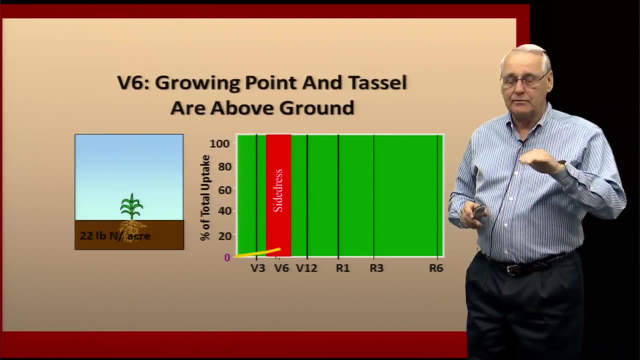 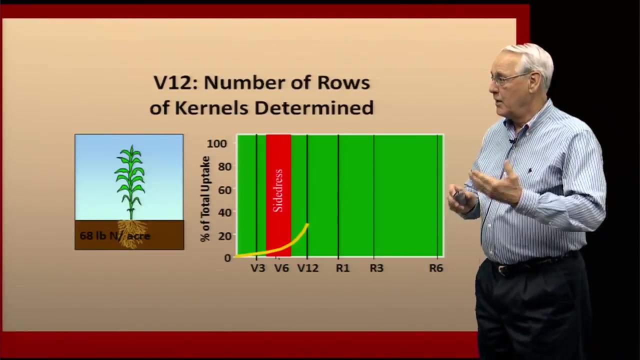 if we're field applying nitrogen fertilizers. But even at the V6 stage we've only taken up about 22 pounds of nitrogen at this time. Now, at the V6 stage, the growing point and the tassel are just about the ground level. At the V12 stage, when the plant has 12 true leaves and is probably 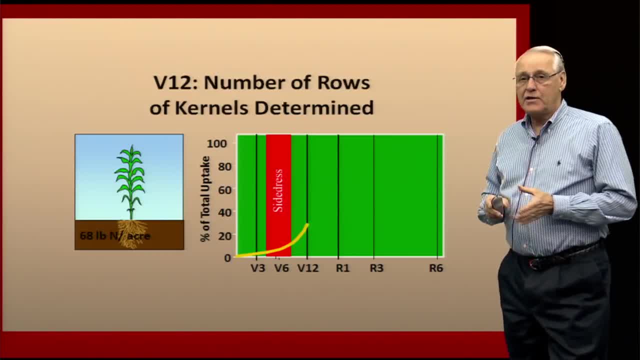 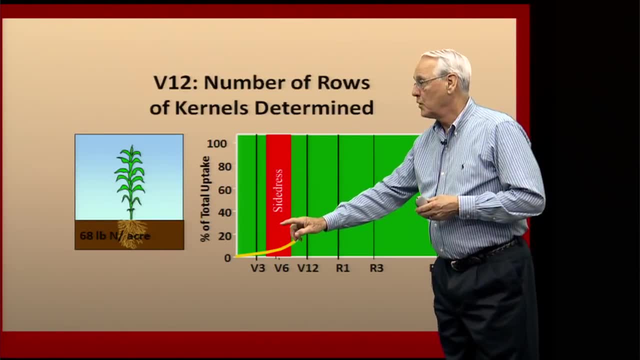 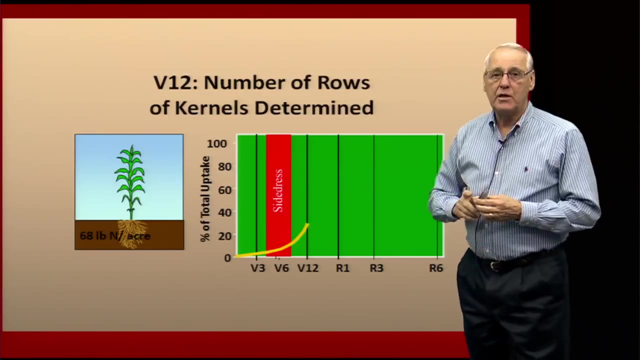 somewhere between four and five feet tall. at that time the number of rows of kernels are determined At that time. you can see, here we're at V12, somewhere between about V8 and V10, we really start into a rapid upgrowth period of the crop. 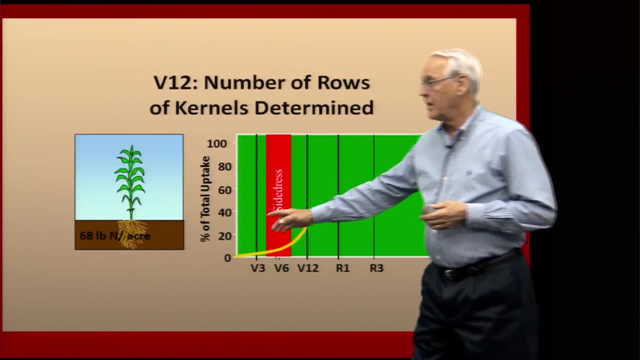 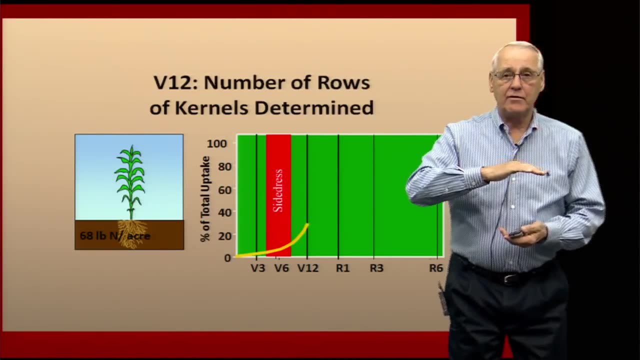 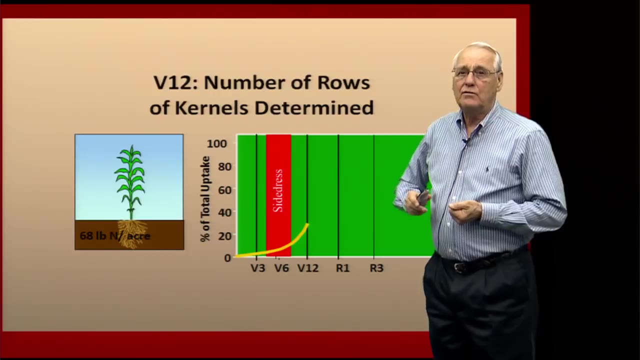 And at that time, by that time, we've taken up about 70 pounds of nitrogen per acre. You can normally think that the amount of rooting that you have in the soil is very similar to the amount of top growth that you have. So when you have about four feet of top growth you've got 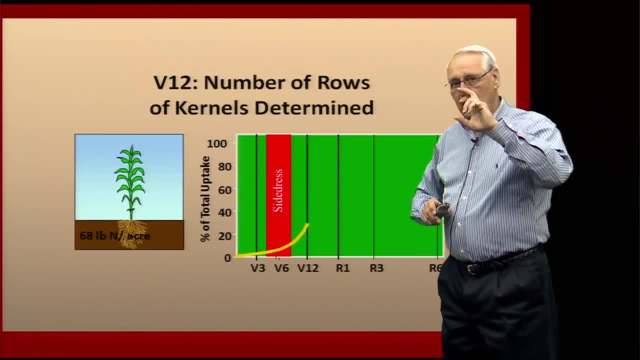 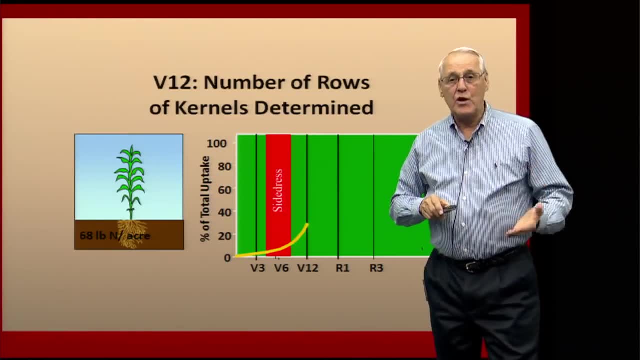 four feet or a little less, of actual rooting. So your rooting is going to develop similar to your top growth. So if you're going to have a crop that's about four feet tall, that's the main root And then from there you start to build a lot more root. Let me explain. 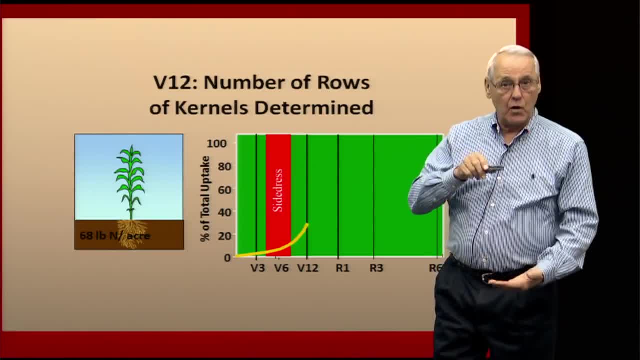 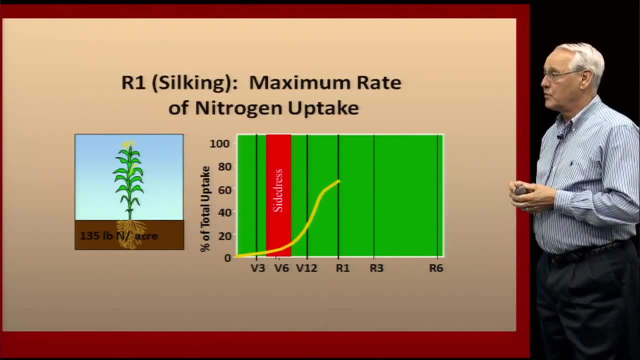 how you can look at the soil in a different light. Now, as you look at the soil, there's a very original rule that applies to all the different parts of the soil. Now if, because we don't have a window into the soil, it's kind of a ballpark rule to say, well, if you look at your 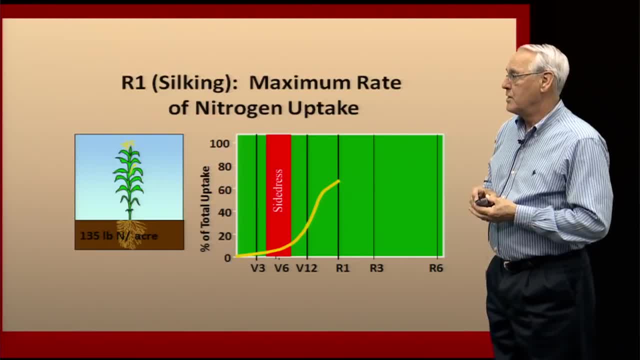 plant growth. you'll have some idea of what your maximum rooting depth is at that time, As the plant continues to grow by the time we get to silking, which is the R1 stage, that's when we have reached the maximum nitrogen uptake. 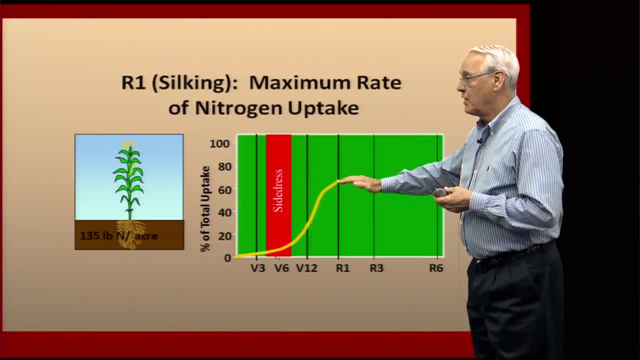 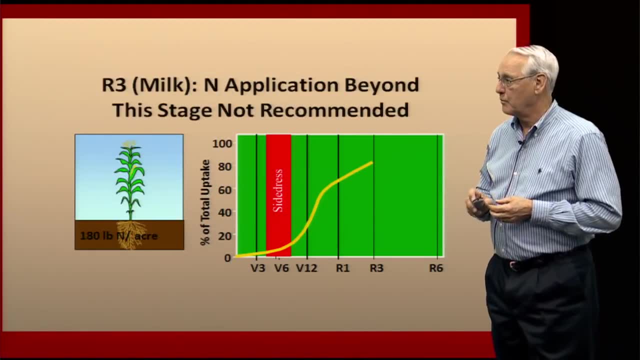 By the silking stage we are up to about a hundred pounds, 60 percent of our total nitrogen uptake. At that time we would have taken up about 135 pounds of nitrogen per acre By the time we get to the milk stage, or what many people call the roasting. year stage of corn, we have taken up almost 80 percent of the nitrogen, And so in this example that's about 180 pounds of nitrogen. Even if you're putting on nitrogen through a center pivot, we recommend that this is a point when you should probably have all of your nitrogen on. 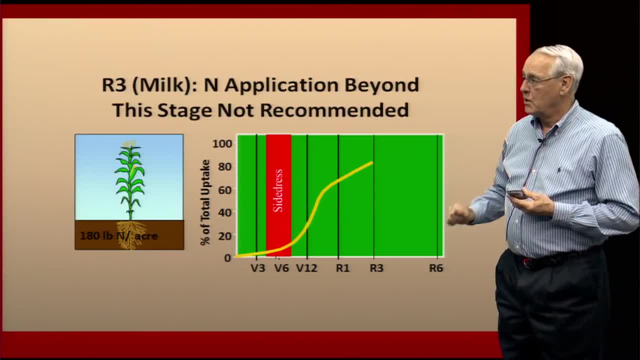 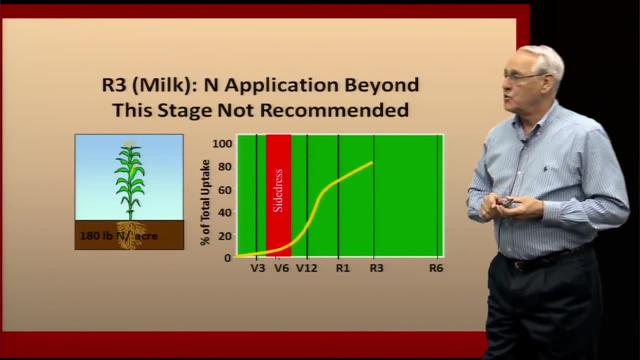 and we don't recommend nitrogen application beyond this stage. You've got your maximum rooting at this time. If you've got most of your nitrogen on, you've got a good root zone that that plant can pull from to take up nitrogen. And if you have a plant that's got a lot of nitrogen on, 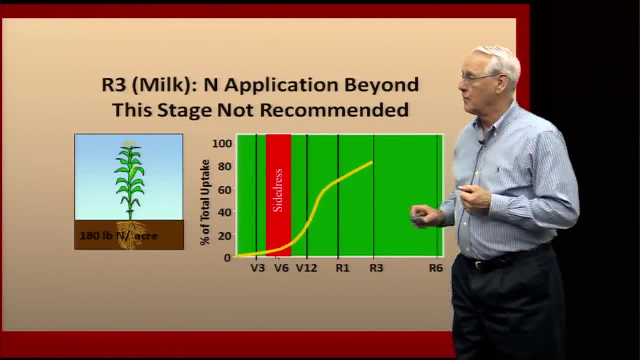 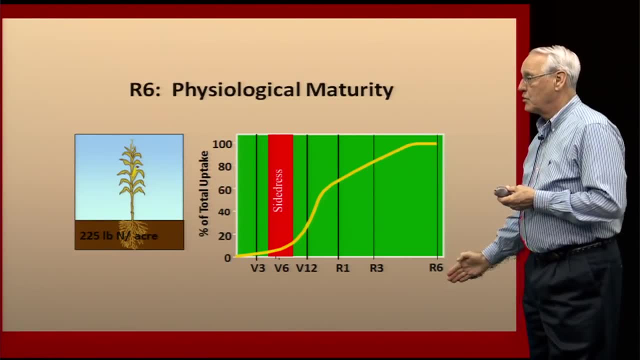 you've got a good root zone that that plant can pull from to take up nitrogen And if you have a proper nitrogen rate and haven't lost any, you should have plenty of nitrogen to finish that crop out to physiological maturity, which is at stage R6. And at that time for a crop that, 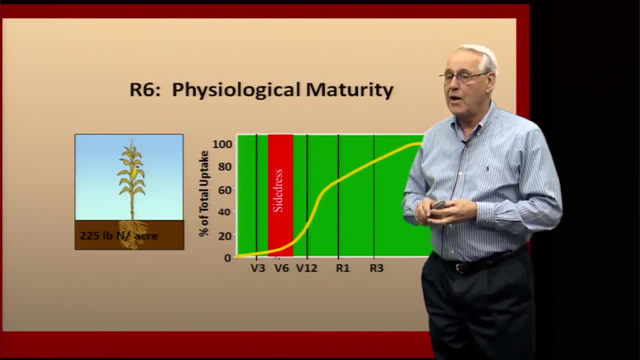 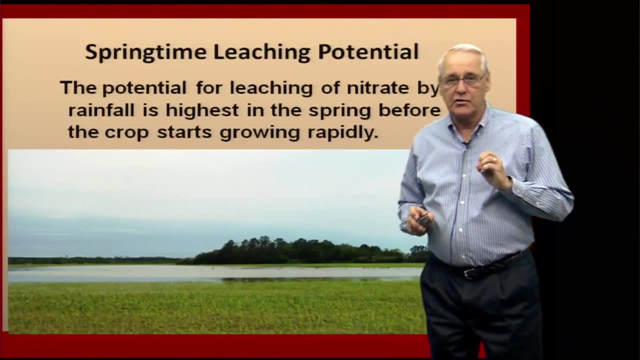 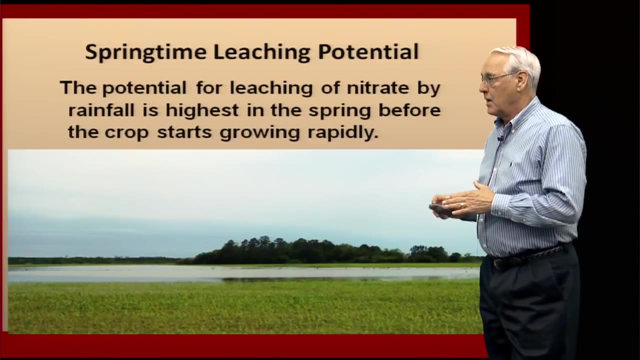 produces over 200 bushels per acre, we will have taken up about 225 pounds of nitrogen. The thing that we want to guard against is springtime leaching potential, because that's really when we lose most of our nitrogen, And the potential for leaching of nitrate by rainfall is highest in the 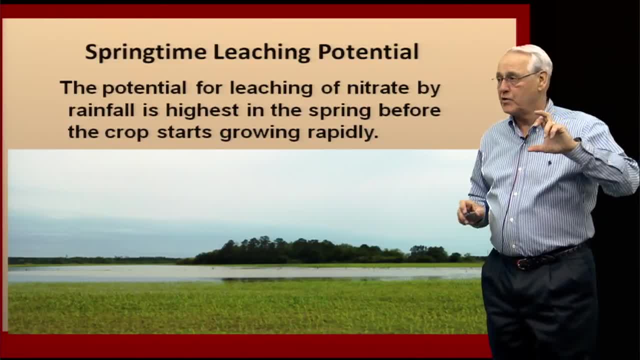 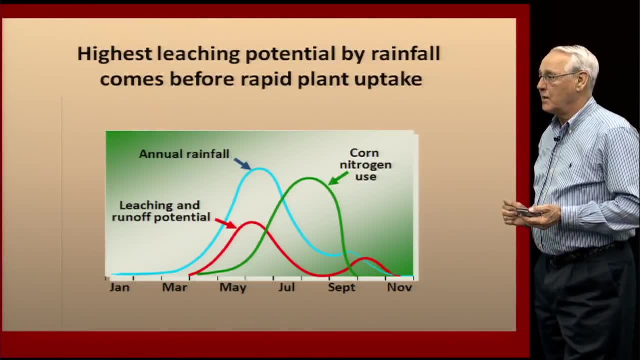 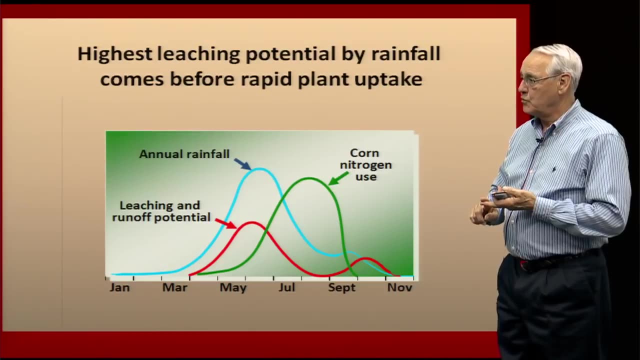 spring, before the crop actually starts to grow and before you have much of a root zone. The other thing, this next slide, I think, gives a good kind of season-long understanding of how plant growth, annual rainfall and crop nitrogen use all come together to kind of define the risk that we have. 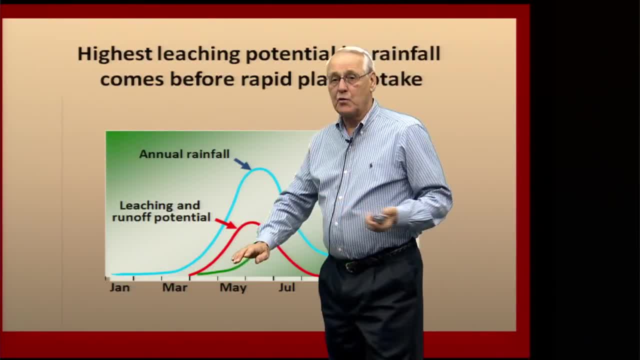 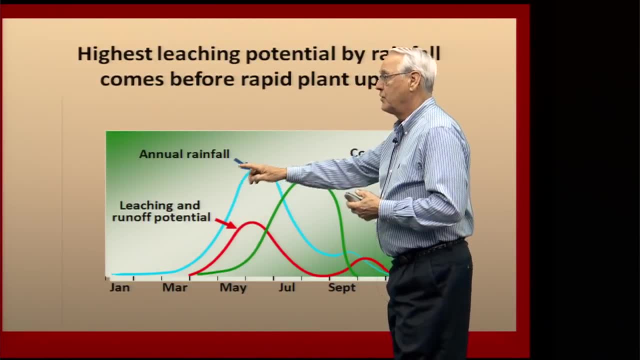 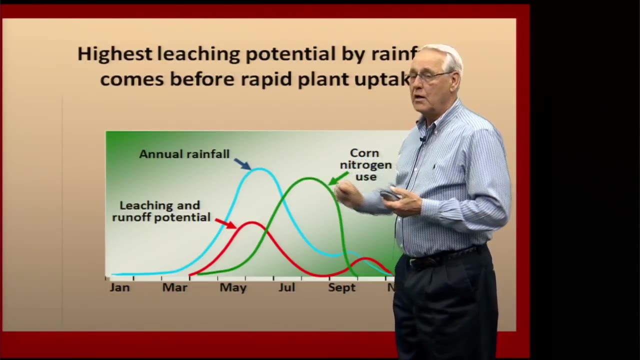 of leaching nitrogen In most of the state of Nebraska. when you go from east to west, we have a rainfall distribution that looks very similar to this pattern. Now, if you're in eastern Nebraska, this peak, which occurs somewhere between May and June, is three to three and a half inches. 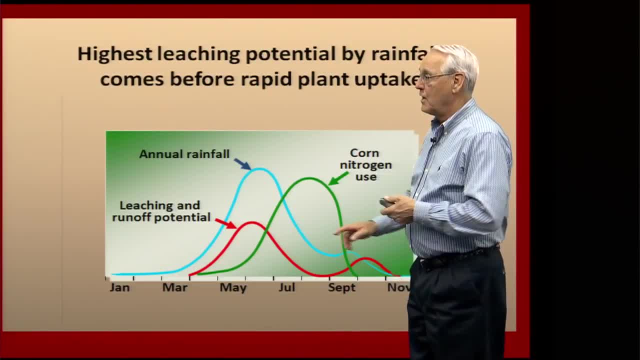 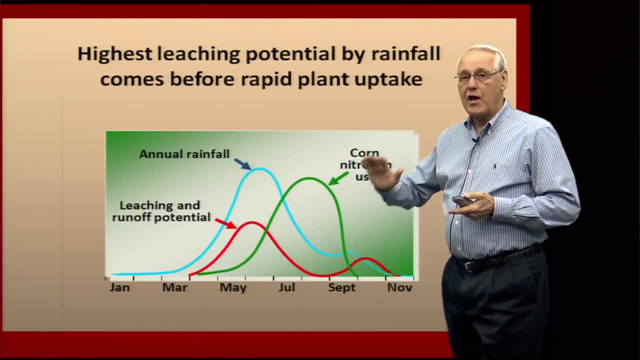 In western Nebraska where we only get 15 inches of rainfall. that peak for the month of June is maybe only two to two and a half inches, But the general shape of that curve is the same: That high rainfall and high precipitation occurs in May, June and the early part of July. 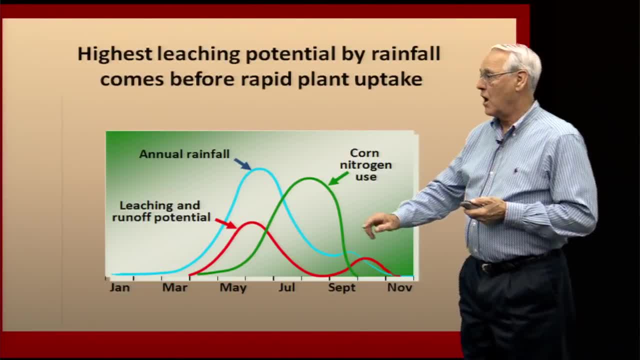 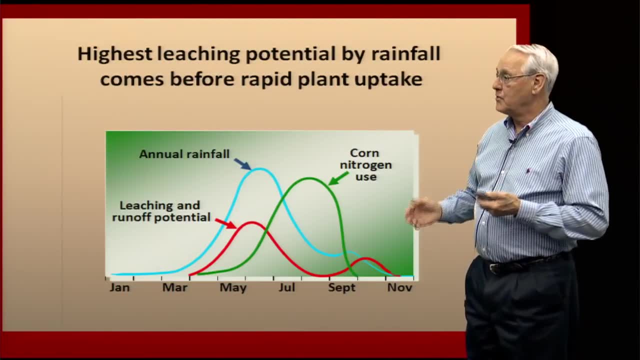 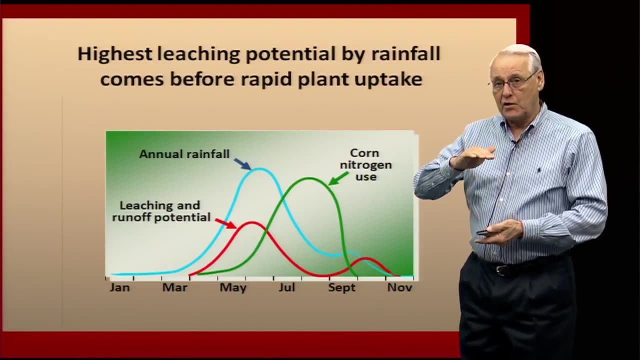 Well, that is our highest period for potential of leaching of nitrogen and also having runoff, Because at that point in the season, if you think back to the developing plant, we don't have a very tall plant. at that time we don't have much of an effective root zone. 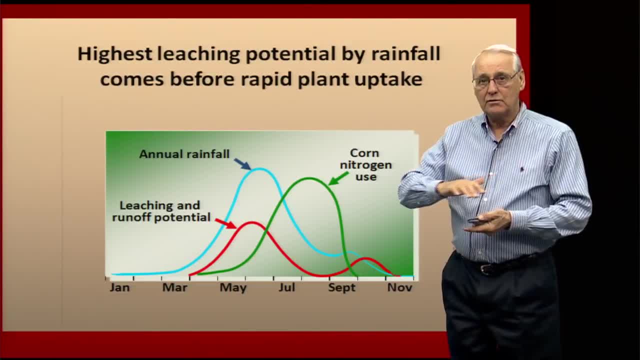 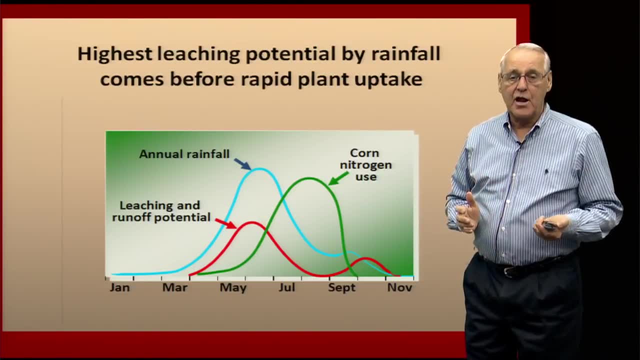 So if we overfill the soil with water and we've got our nitrogen there and we move water, that water is going to move that nitrogen, primarily nitrate, down with the wetting front of the soil. Now, if we don't oversaturate, 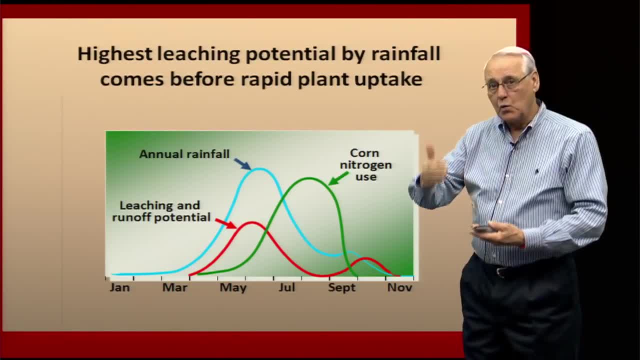 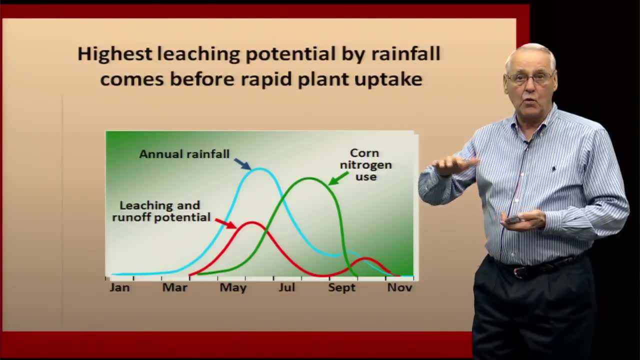 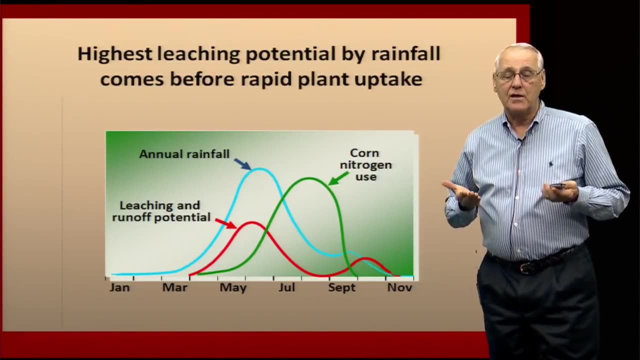 that soil and we capture that in the effective root zone. we can catch that nitrogen later as the plant roots grow. but if we continue to have rainfall or we over irrigate, we continue to move that nitrogen down through the soil and eventually we will get it beyond the effective range of the 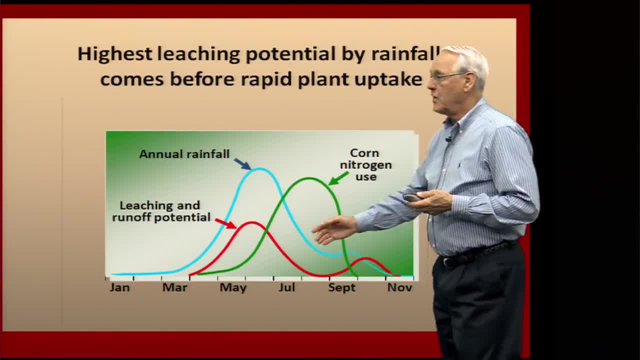 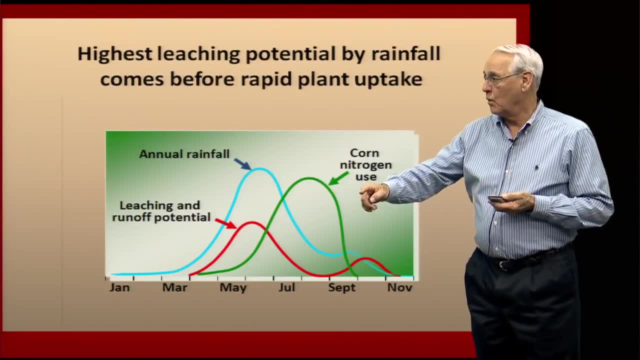 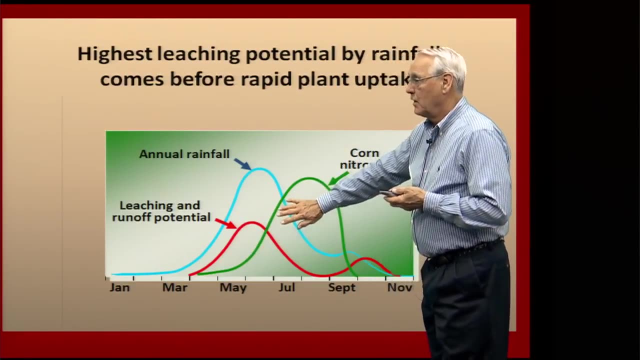 root zone and we will not be able to recapture it. So in this example the rainfall comes early. our main crop and nitrogen use come later in the season. So really, if you remember, when we were talking about the nitrogen update that occurs really pretty much, starting quite rapidly. the 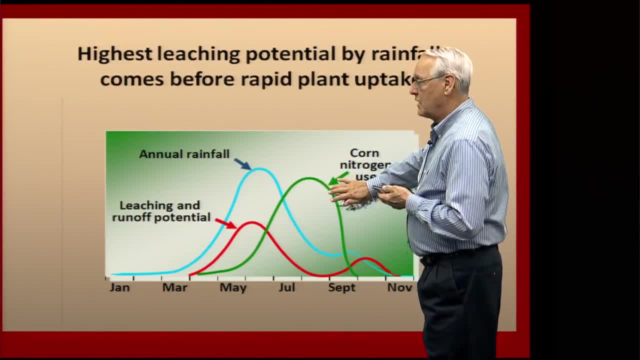 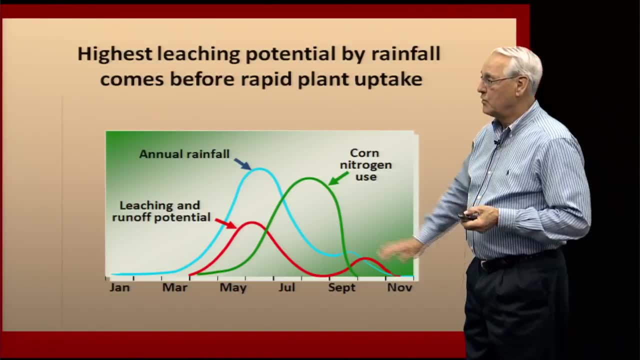 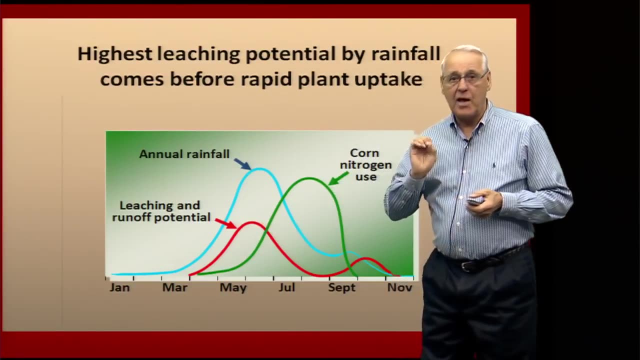 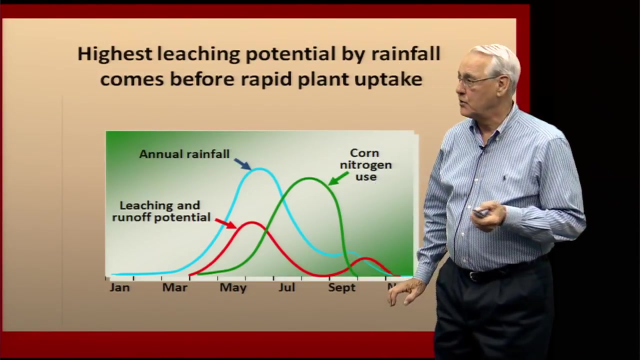 first part of July up through August it tapers off a little bit, but even into September we have quite a bit of nitrogen uptake and also water use. So managing our water in the early part of the season and managing our nitrogen from the standpoint of timing are two keys to making sure that we don't lose and leach. 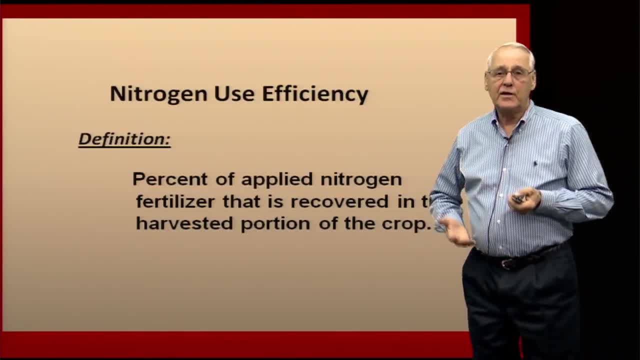 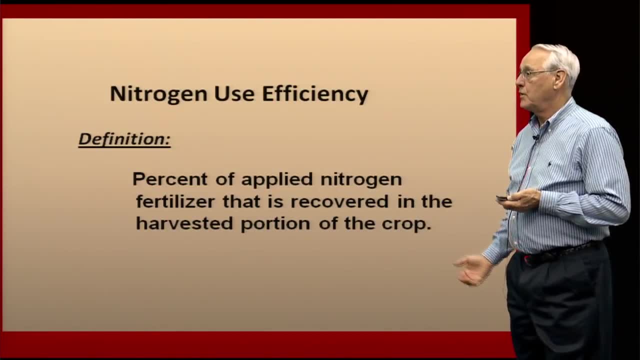 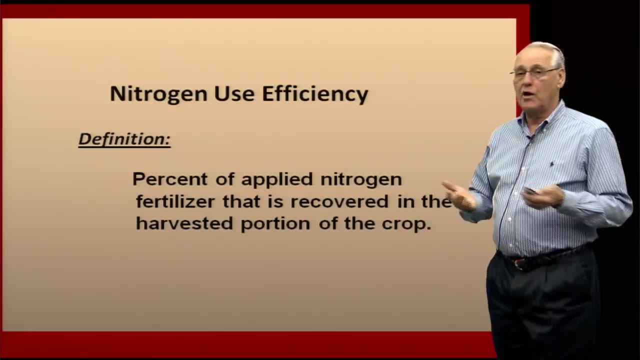 that nitrogen. When we effectively use nitrogen, we just have a term we call nitrogen use efficiency, and nitrogen use efficiency is simply the percent of the applied nitrogen fertilizer that's recovered in the harvested portion of the crop. And many times if we're harvesting grain we're leaving the stover. but really looking at the amount of 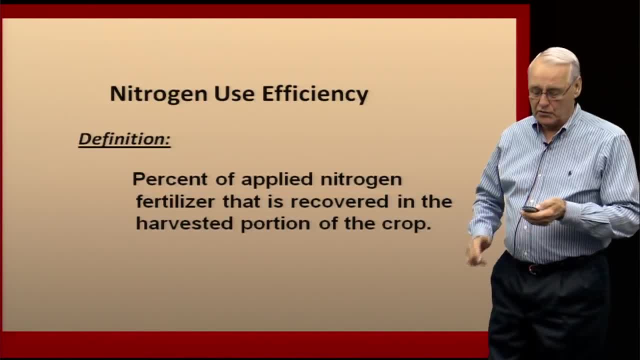 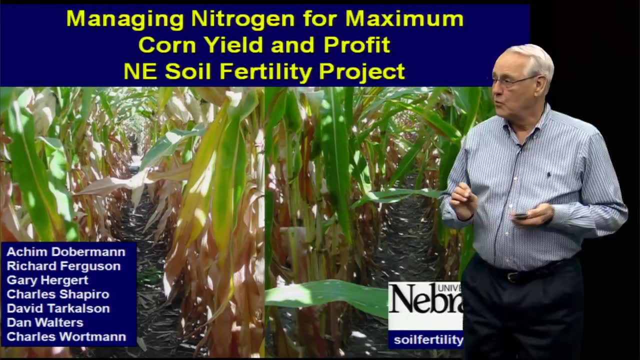 nitrogen that we took up in the stocks and also the grain. One of the more important things that we've done over the years in Nebraska is we've spent a lot of time in the forest for fruit to be able to take in the plant to grow. We've used, and that, I think, is the most effective. 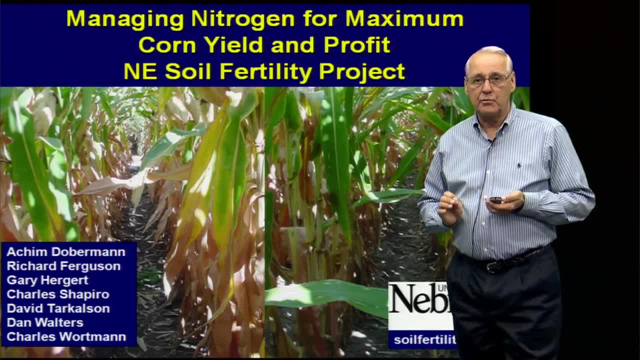 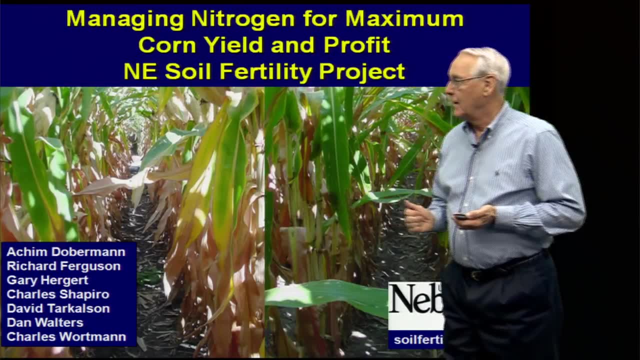 approach to making sure that we have the right amount of nitrogen and we can use it in the future: a lot of research and time on trying to improve our nitrogen recommendations, for corn Corn is the biggest nitrogen user of all of our crops in the state and we've done a number. 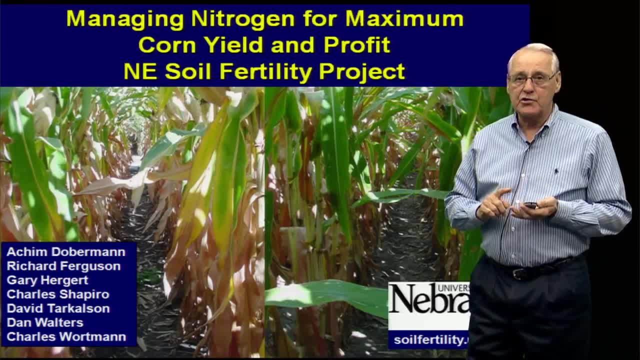 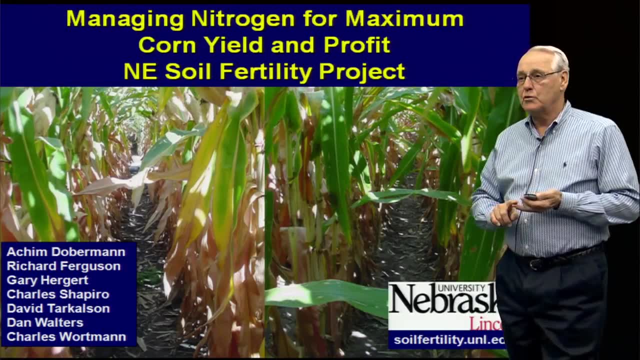 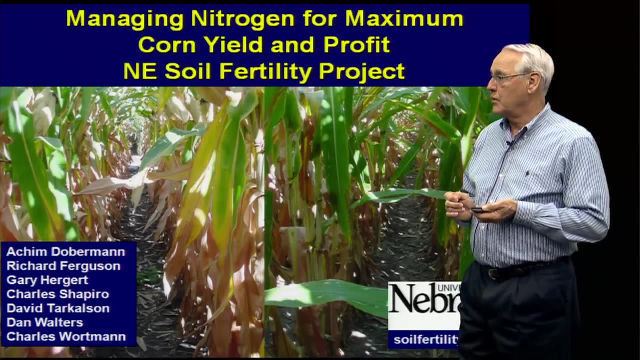 of experiments to look at nitrogen rates and nitrogen timing at corn to get maximum profit but also to have the best nitrogen use efficiency. Back in the early 2000s we redid a series of nitrogen rate studies called the Nitrogen Soil Fertility Project. A number of us were 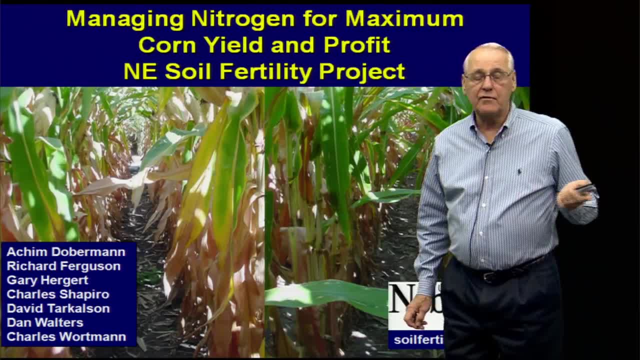 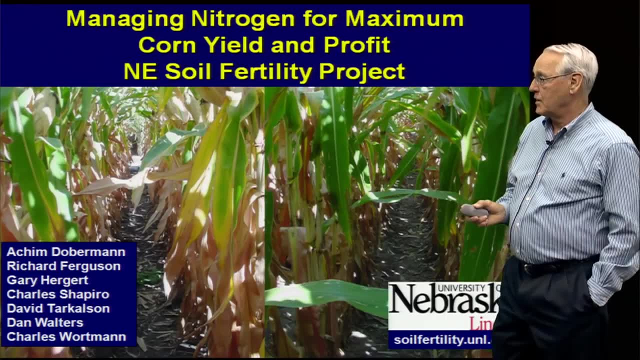 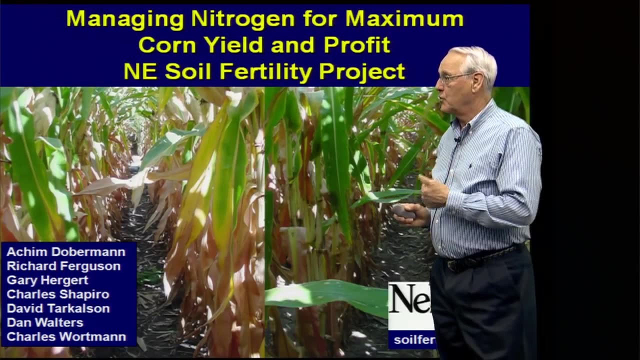 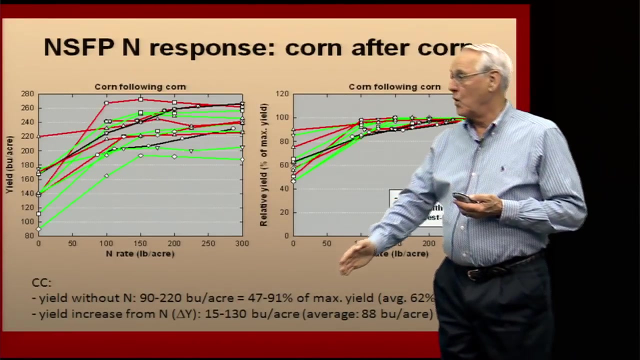 involved in this where we had locations across the whole state of Nebraska at a whole range of fertilizer nitrogen rates. when we were trying to see about how we could, if our nitrogen recommendations were adequate for the new higher yields we were producing, and also how we did in terms of our residual nitrate, We had nitrogen rates that went all the way up. to 300 pounds per acre, which no one would use these days. but actually back in the 1970s, when anhydrous ammonia was very cheap, we had a lot of farmers then when they were producing 150 bushels of corn who were putting on 200 to 250 pounds of nitrogen. So through these, 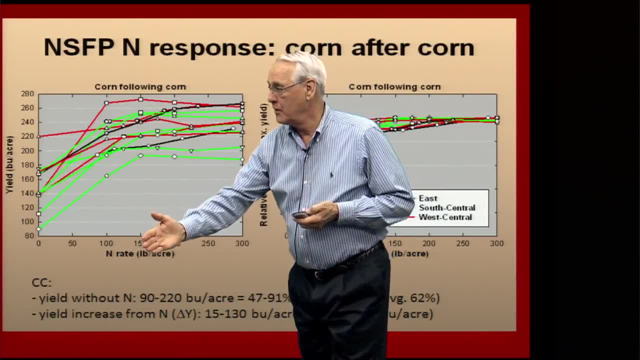 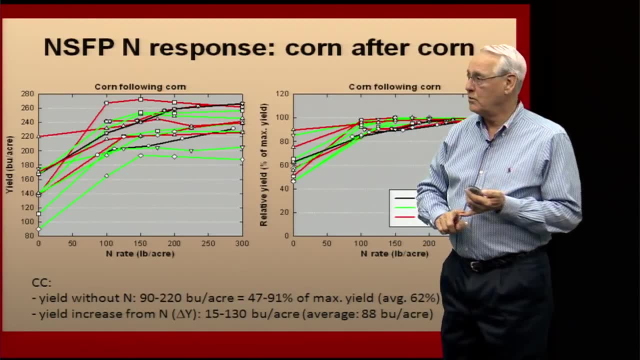 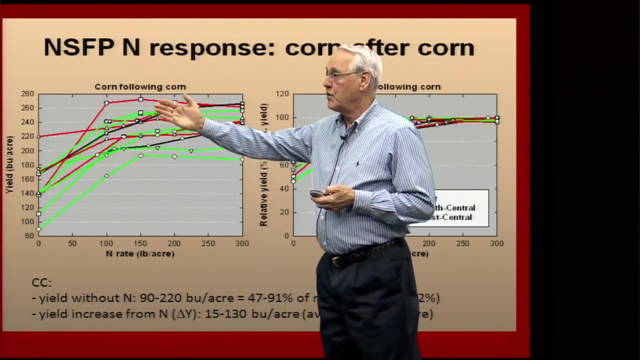 experiments. what we did. we put on nitrogen rates in 50 pound increments. then we would create a yield response function. We did this for continuous corn or crop yield response for corn after corn. The data on this slide just shows the actual yields We had check. 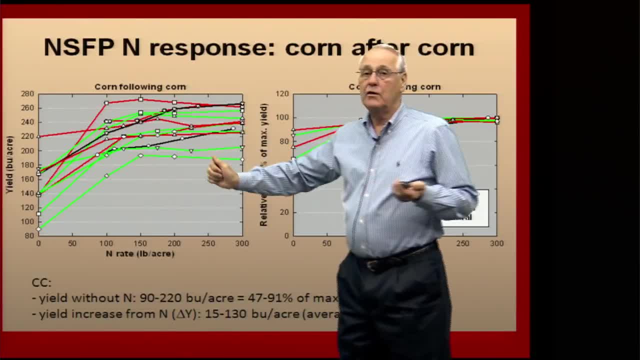 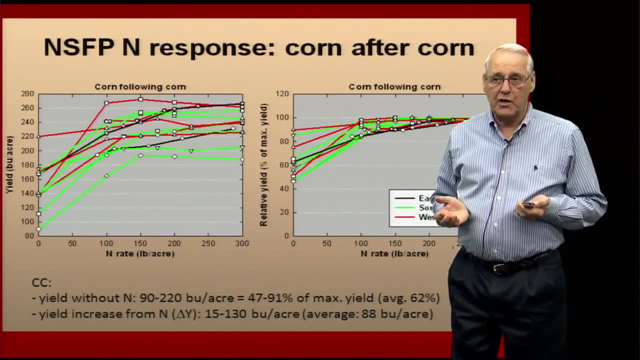 yields from as low as 80 bushels. We had corn plots that yielded up to almost 270 bushels per acre. In our earlier data set that we used to develop our nitrogen recommendations, our yields 20 years ago were maxing out at about 200 bushels, So we really needed a data. 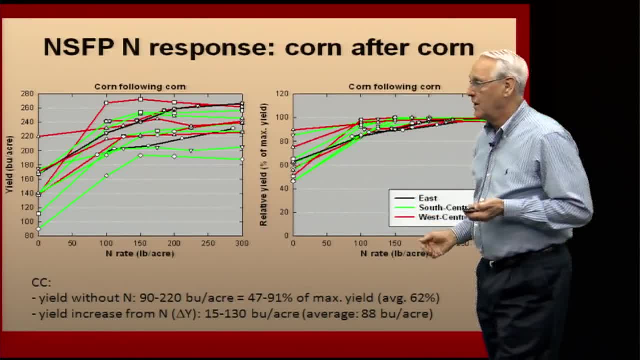 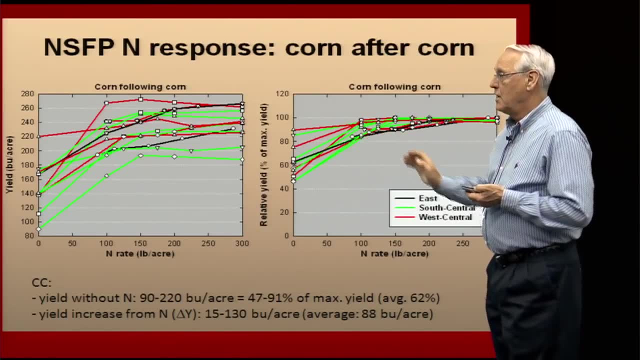 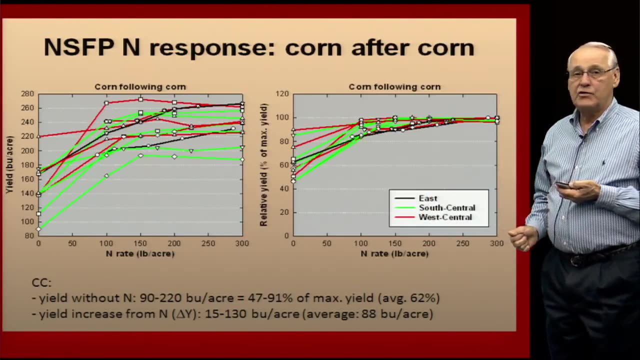 set that reflected the higher yields that we're producing today. We can translate those yields into a relative yield. When we do that, it takes out some of the variability. but taking if we look at corn after corn, the different colors represent the different areas in the state, What we found in some places if we had high residual nitrate, we didn't get much of a response to nitrogen. Generally, however, if we applied no nitrogen, we had yields that ranged from as low as 90 bushels per acre. So we had a yield that ranged from as low as 90 bushels per acre up to 220.. If we averaged all of the sites and over time we did about 35 sites across the state. our average yield without nitrogen was about 62% of the maximum yield And that's generally. what we find is that, if you put on, if you've been fertilizing a field following normal farming practices. 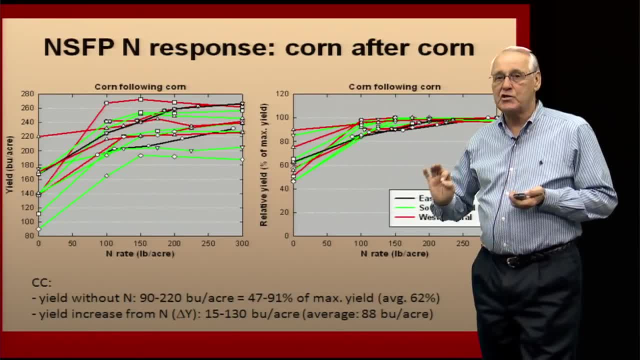 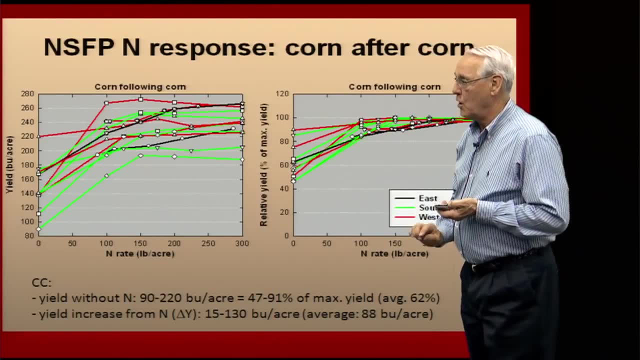 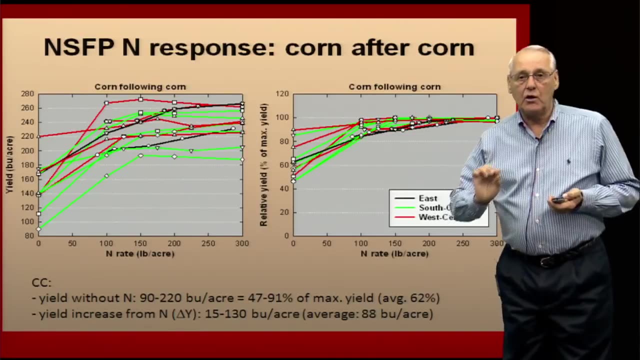 if you plant a crop the next year and put no nitrogen on for corn, you'll get about a 60% of your average yield. Now the yield increase that we got from the nitrogen that we put on ranged from only 15 bushels an acre up to 130. But in general, on corn following, corn. when we applied a proper rate of nitrogen, we generally had a difference between the check and the response of about 90 bushels per acre. We also did this for corn following soybeans. What we found with corn following soybeans was that with no nitrogen, we yielded all. the way from 105 to 210 bushels per acre. Our average yield of corn without any nitrogen, following soybeans, was about 72% of the maximum yield. Now, if you remember, on the previous slide that was higher For continuous corn, that number is only 62%. 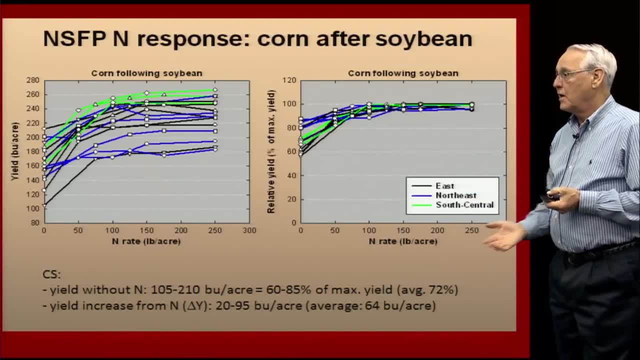 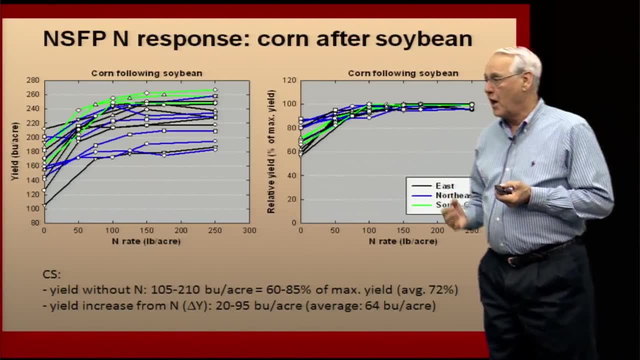 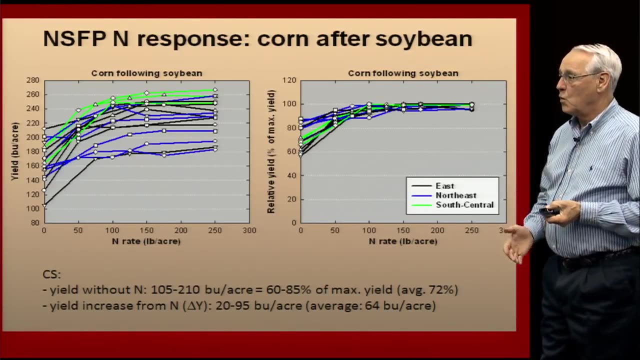 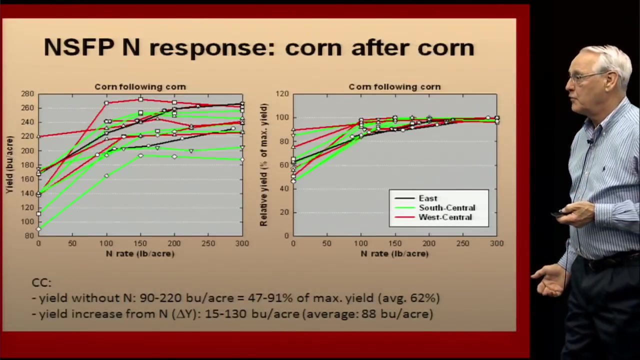 So we know that soybeans do fix some nitrogen and we're seeing that reflected in a higher check yield with no nitrogen. The yield increase that we got from nitrogen applied to corn following soybeans was 20 to 95. Our average yield increase was about 64 bushels per acre. 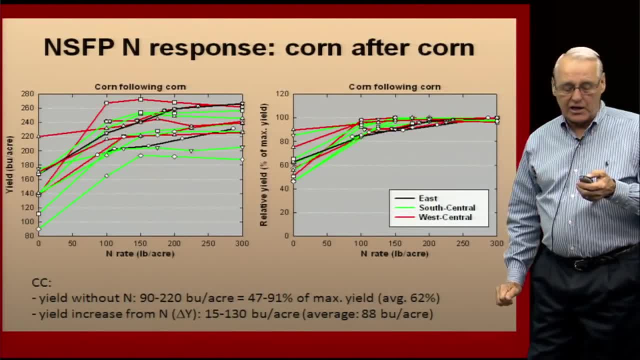 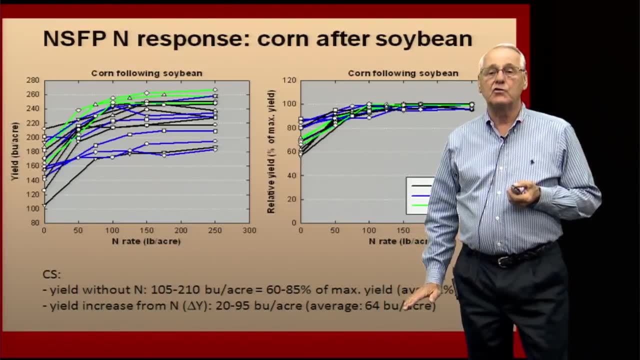 If you remember, when we were corn following corn, it was 88. So this is a good example of how we're going to do this. We're going to go ahead and do a good indication that we are getting a nitrogen effect from those soybeans. We do have a soybean. credit that we give when we make our nitrogen recommendations of about 45 pounds. That's kind of an average. You can see if we just take the difference here between 64 and 88. it's maybe a little less than that, but in most cases we feel the 45 is a pretty good. 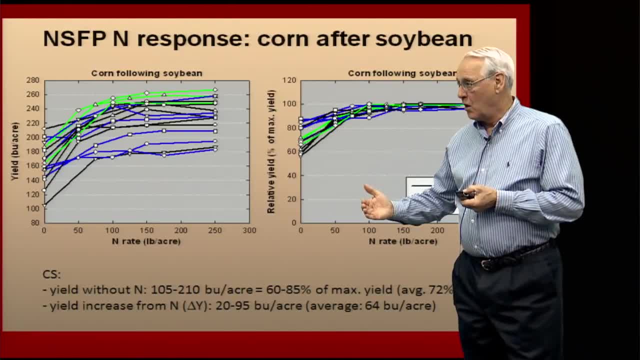 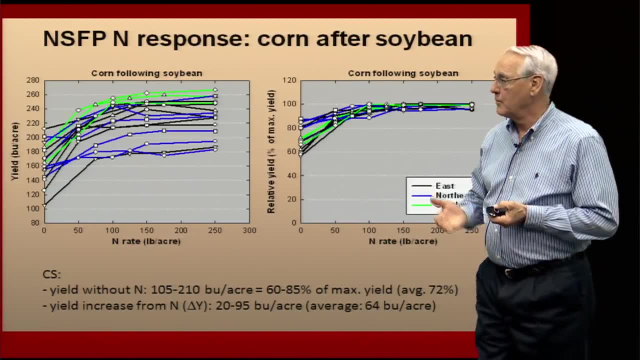 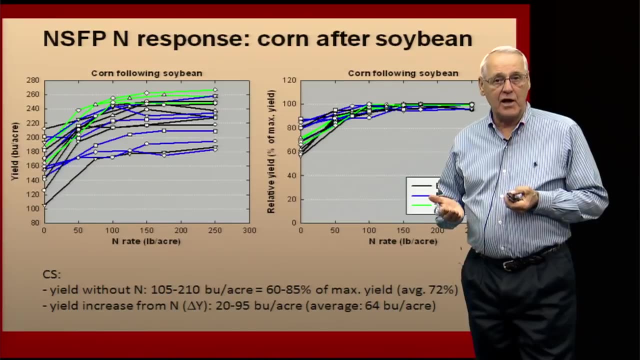 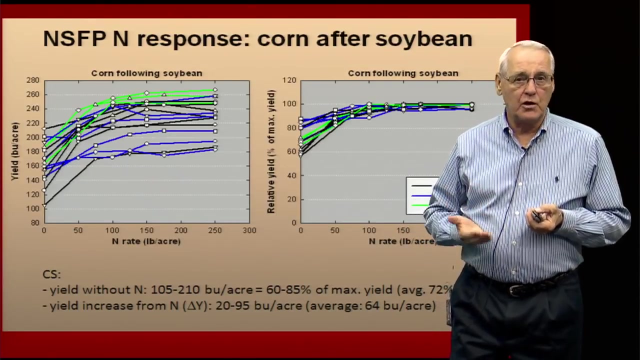 value. With that, all of this data, We use these values in our nitrogen recommendation algorithm and we found that the equation that we use still is a very good predictor for the amount of nitrogen that we need for today's higher corn yields, when we have a lot of producers that are hitting 230, 240 bushels per acre. 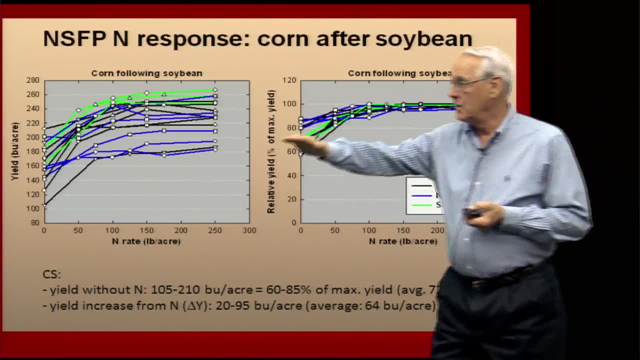 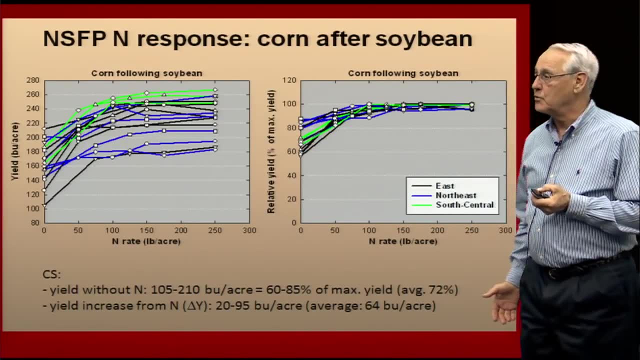 sometimes even 250. And we have a data range in this data set where we produced up to those high yields in our plots. We were producing up to a lot of corn yields in our plots. We were producing at the maximum 260 to 270 bushels per acre. Now, whenever you apply nitrogen, 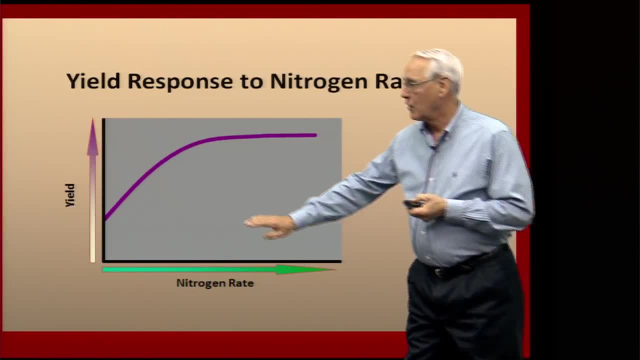 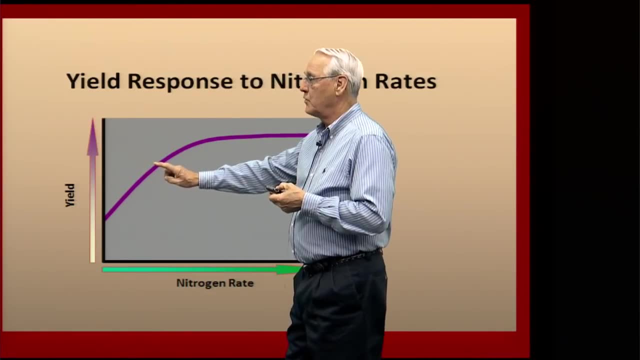 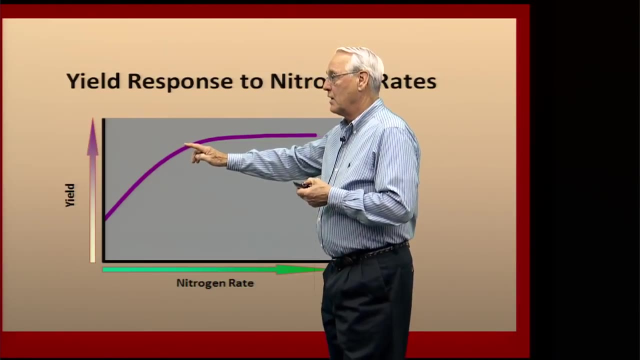 to growing corn, you get what we call a curvilinear response. So you have a yield. you have an almost linear increase. but then as you continue to add nitrogen, the yield that you get for every additional pound of nitrogen begins to decrease And it's kind of a diminishing. 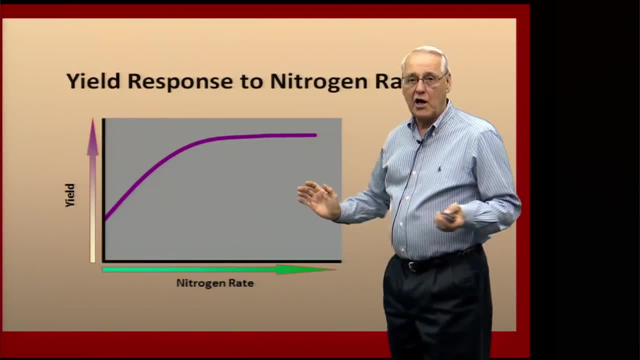 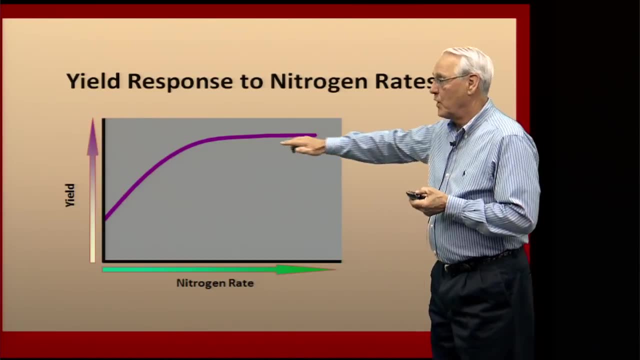 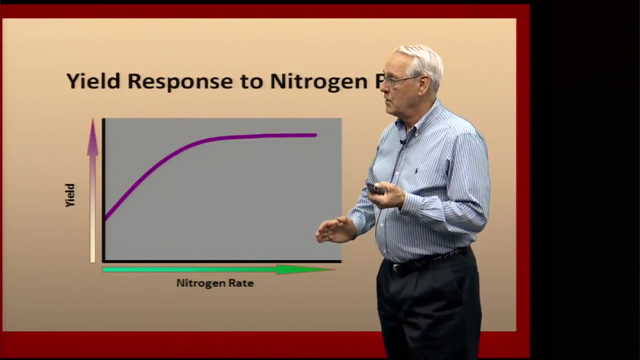 return 19, a lot of nitrogen to today's hybrids. Back when I started with the university, when we went out to these high nitrogen rates, we actually saw this curve tail off. We had lodging, we had stock quality problems. Today's newer hybrids will stand higher nitrogen rates but 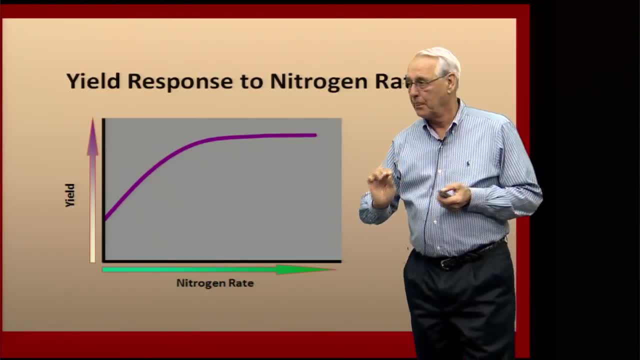 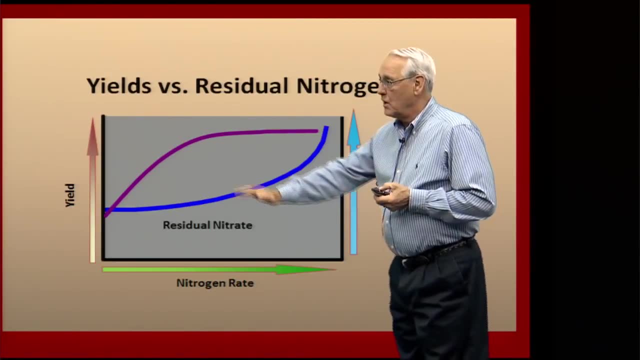 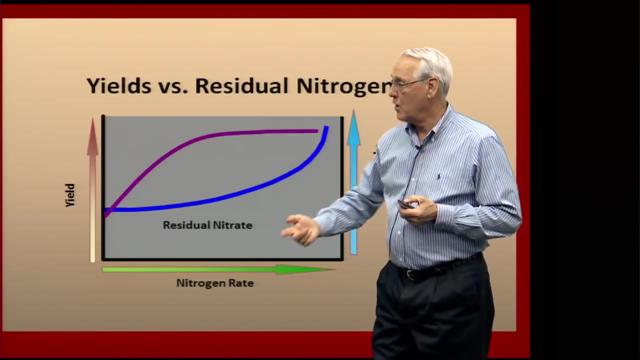 that doesn't give us any yield increase and it causes some other problems, And that is any time we fertilize corn with nitrogen in addition to the yield curve, the thing that we don't see if we go into these plots and soil sample after the crop is gone. we 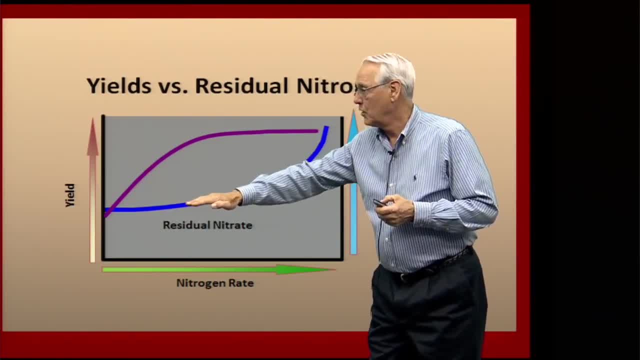 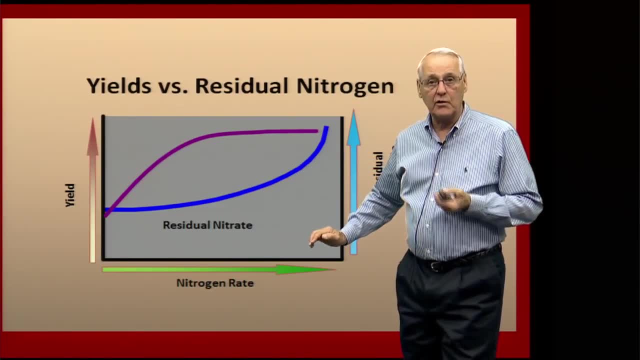 will see that the residual nitrate level has a curve and that as we increase nitrogen rate, we also increase the nitrogen that we leave in the soil, the unused nitrogen. What we find is that once we hit the point of our maximum yield, we're going to see that the 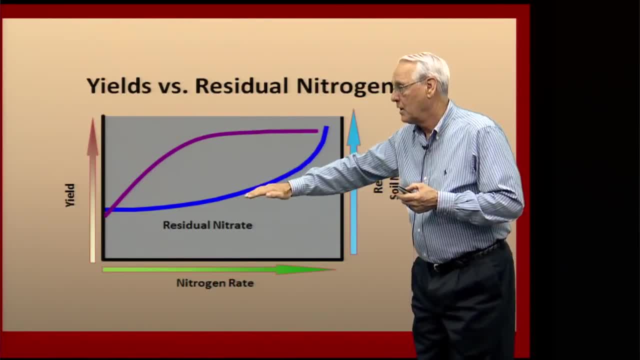 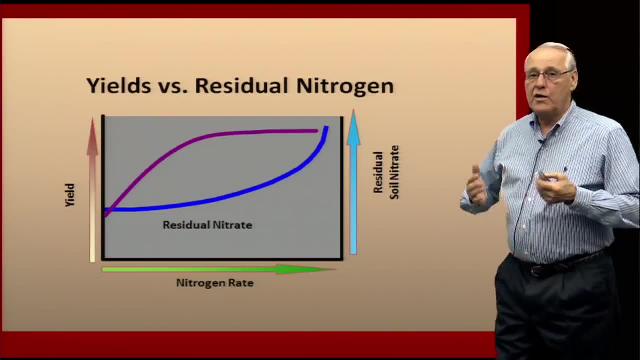 maximum yield, which in this case would be somewhere back in here. Then that nitrogen, that residual nitrate, really begins to go up. So we know that if we over fertilize we may not suppress the yield of the crop but we will greatly increase the residual. 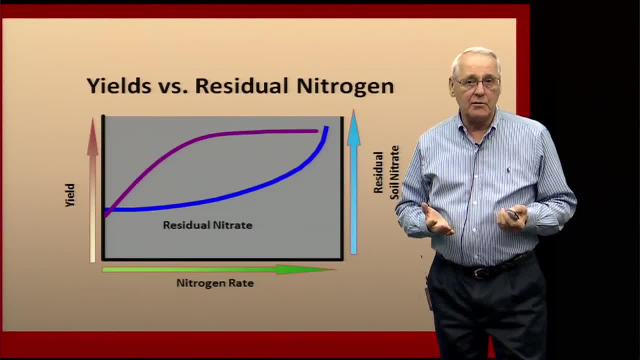 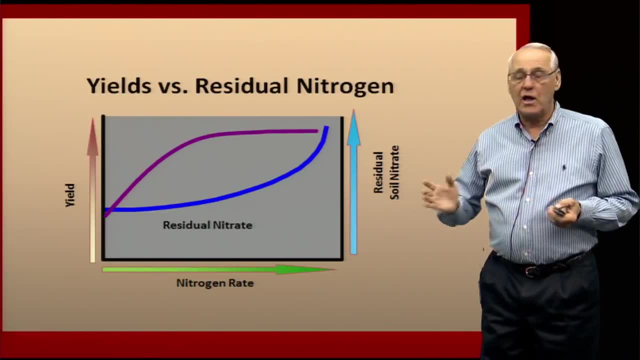 nitrate in the soil. Now, if we're in a drier climate, we can recapture that nitrogen in the next crop if its not too deep in the profile. But in a wetter climate, if we leave a lot of nitrogen in the soil, we have the risk of losing that nitrogen. 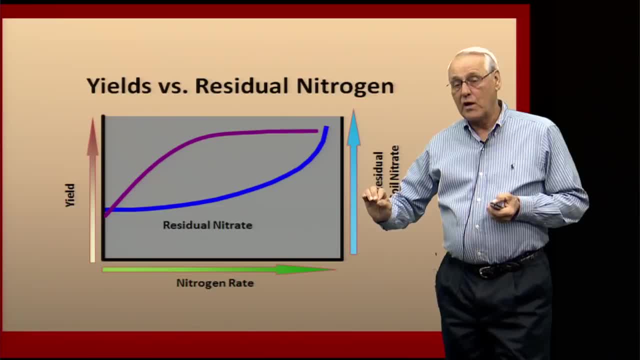 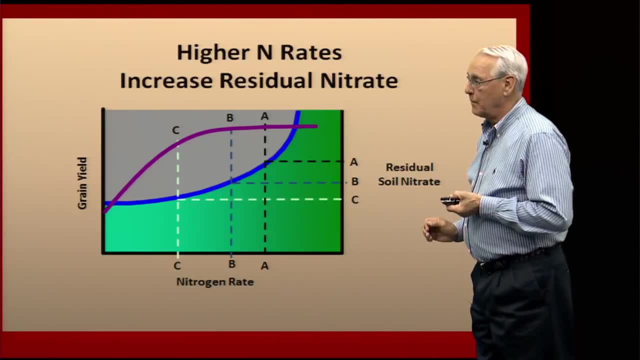 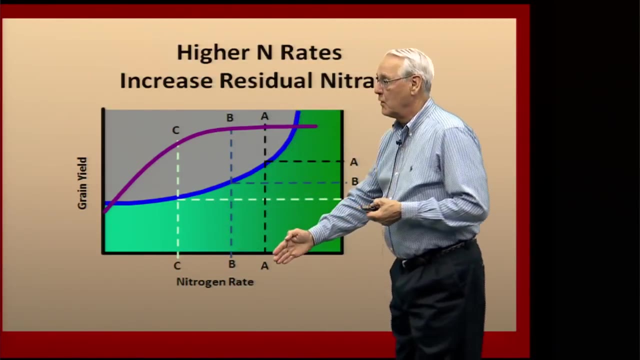 if we have high rainfall the next spring and the soil is wet. So if we take this curve and we look at some different points on it- I've just taken three points on here and I looked at nitrogen rates C, B and A- We take those up. 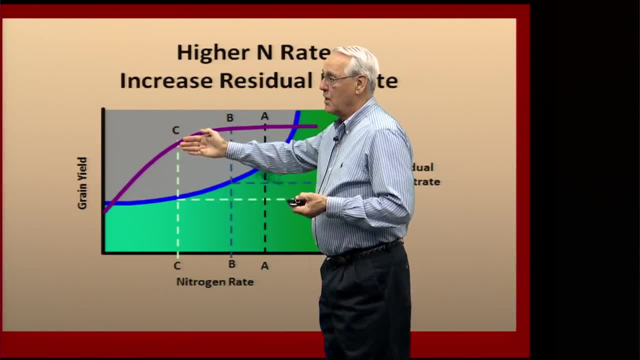 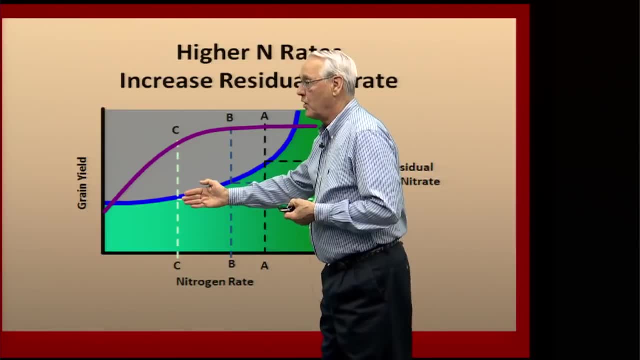 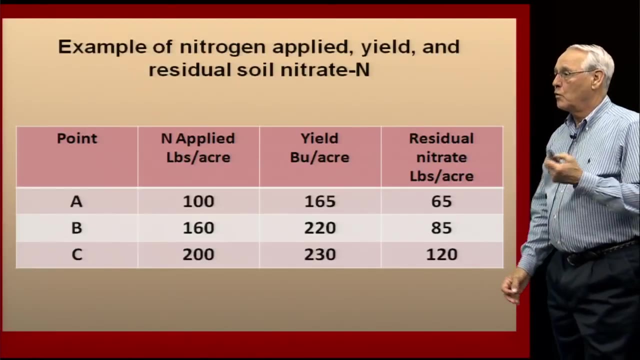 We're going to show you the yields at point C, B and A. We're also going to show you what you have as residual nitrate at point C, B and A. So in a scenario where we're producing about a 230 bushel, 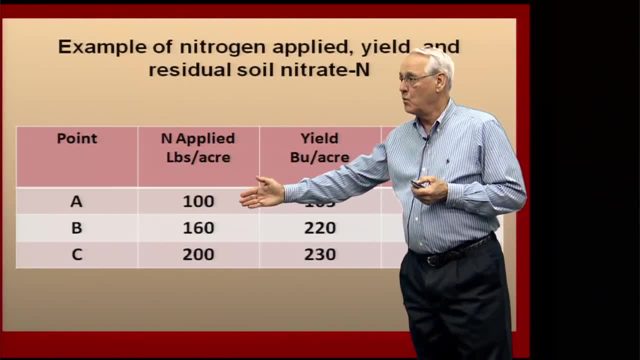 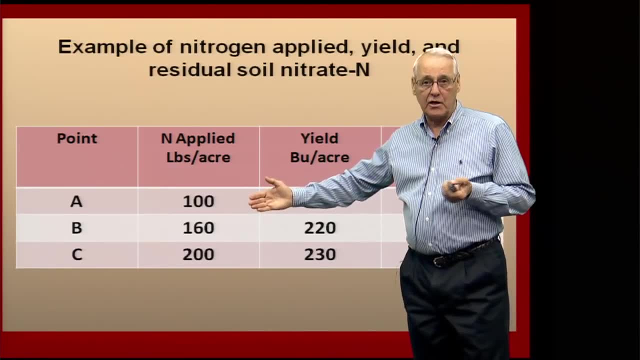 corn crop. at point A, we applied 100 pounds of nitrogen, And this is very typical of the data that we saw from that NSFP project that I showed you earlier. At 100 pounds of nitrogen, we produced 165 bushels of corn. 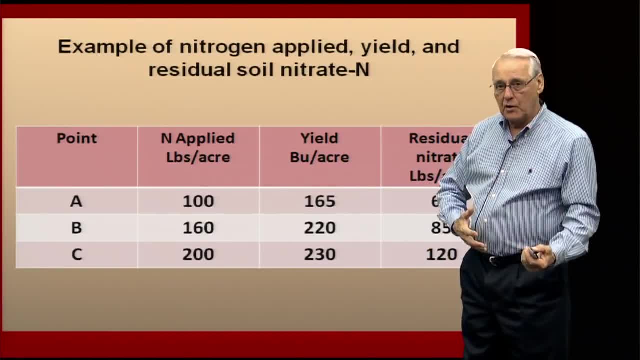 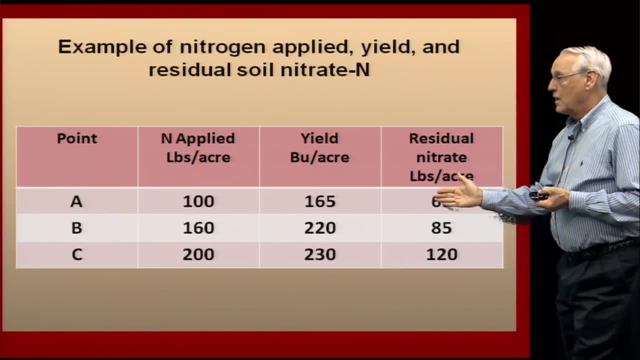 Our hybrids today have very good rooting systems. They use the mineralized nitrogen, They use the fertilizer. We're getting great nitrogen efficiency but we're not maximizing our yield At that low level of nitrogen. we still have some residual nitrate. 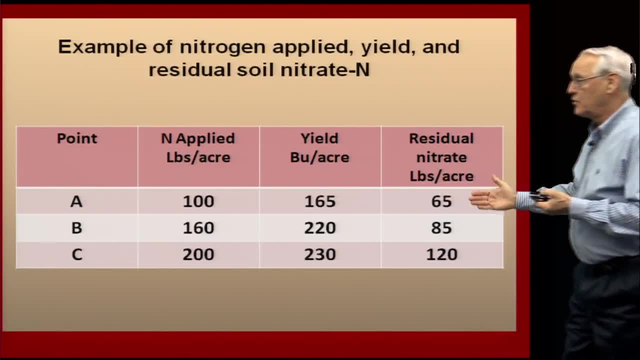 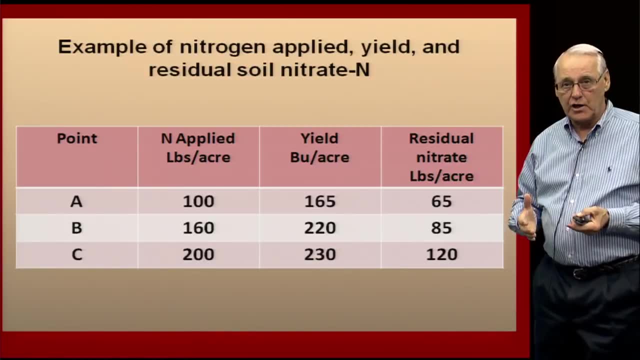 If we would have put no nitrogen on, we would still see residual nitrate, probably a low level. It's a low level of 25 to 30 pounds, but there's always some residual nitrate there in the soil. At point B on the curve, that was where. 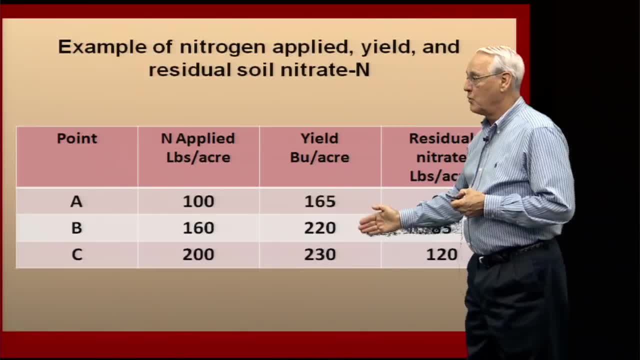 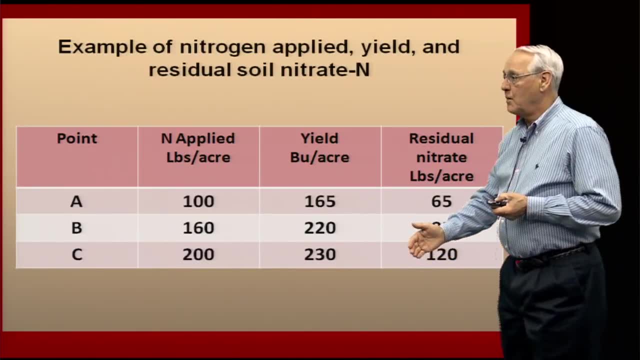 we would apply 160 pounds of nitrogen. We produced 220 bushels per acre And our residual nitrate does increase, but it doesn't increase rapidly. If we applied up to 200 pounds of nitrogen, we did get, in this example, 10 more bushels. 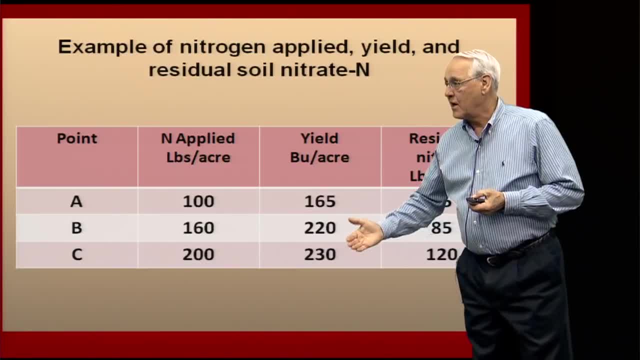 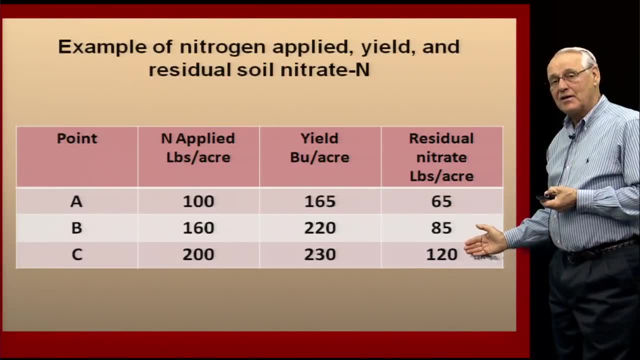 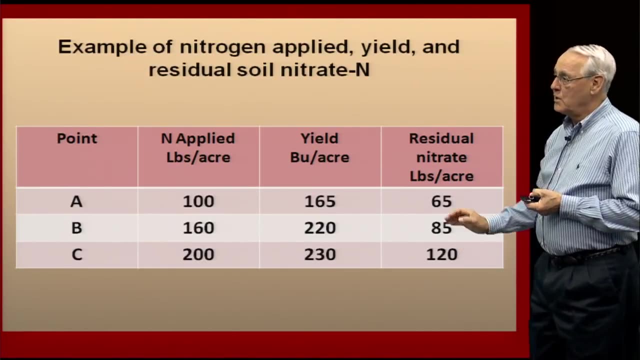 But we weren't using that nitrogen very efficiently And that extra 50 pounds or 40 pounds of nitrogen actually showed up that we had 35 pounds of that that remained in the soil and we had 120 pounds of residual nitrate, And so we need to look at where we're. 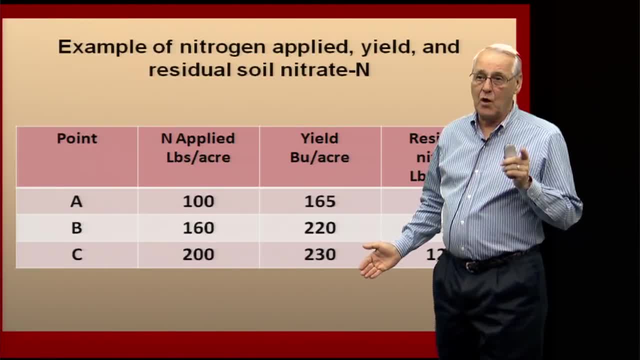 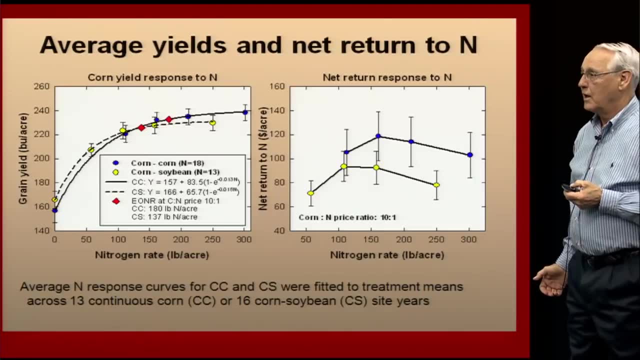 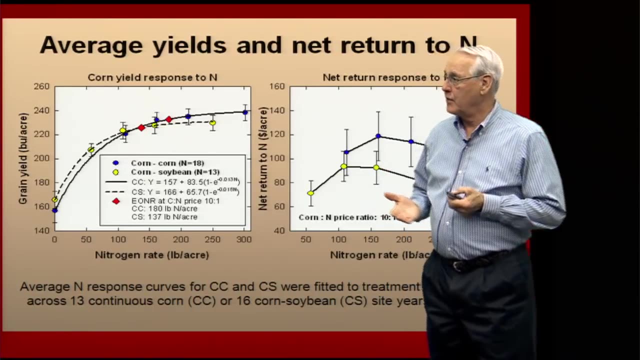 going to get our maximum yield- not necessarily always our maximum yield- our maximum economic yield and what we're doing in terms of the residual nitrate that we're creating in that soil. As we looked at our average yields across that NSFP study. and our average return to nitrogen. we generated curves where we looked at the grain yield for the continuous corn and corn following soybean, The corn following corn: we had 18 site years of data. For the corn- soybean: we had 13 site years of data. 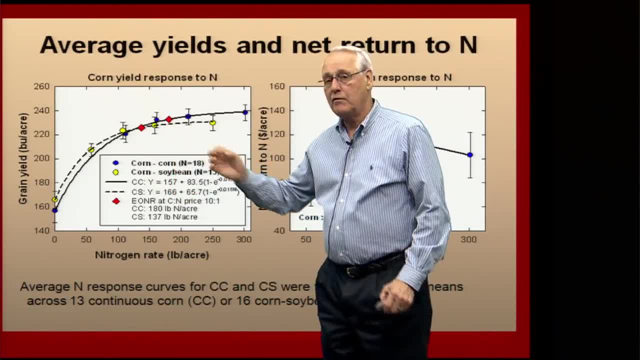 We developed a mathematical equation to define that curve. When you do that, you're going to get a lot of data, And you're going to get a lot of data. And you're going to get a lot of data. And when you do that, you can do some mathematics. 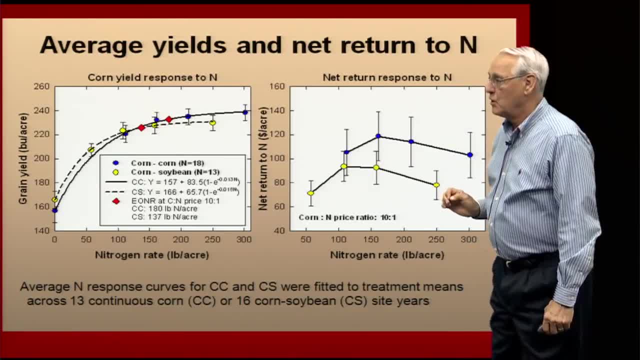 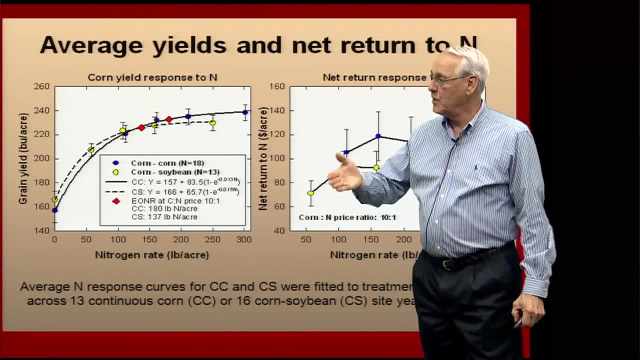 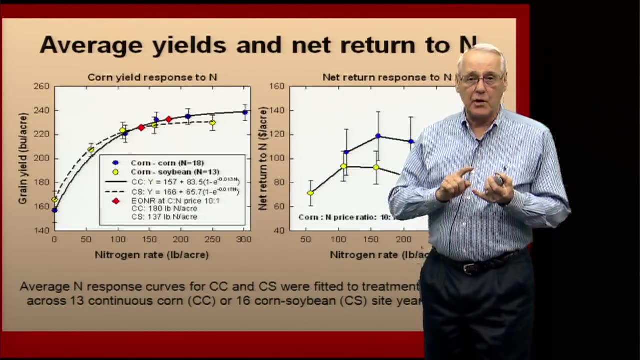 to determine when you got the maximum net return to your nitrogen And what we did for the corn following corn and corn following soybeans. we used those equations, we did the mathematics and we could determine then, based on the price of corn and the price of nitrogen. where the most economical point was Not necessarily the most The maximum yield, but the most economical point in terms of the profitability of the nitrogen that you put on. And generally what we find is the most profitable point is usually a little bit lower than the maximum yield. 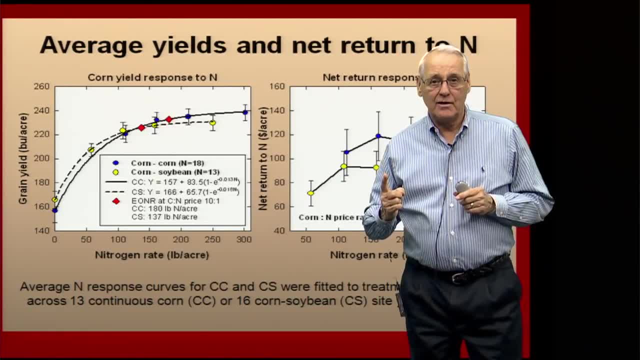 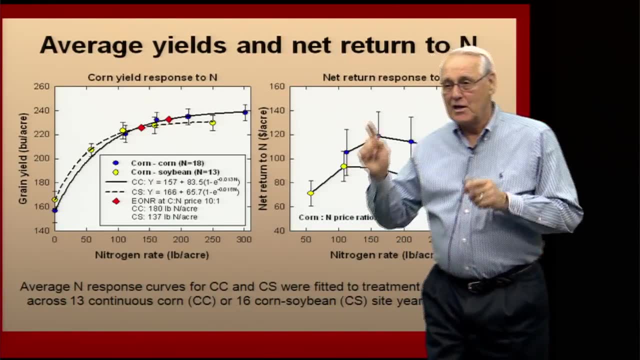 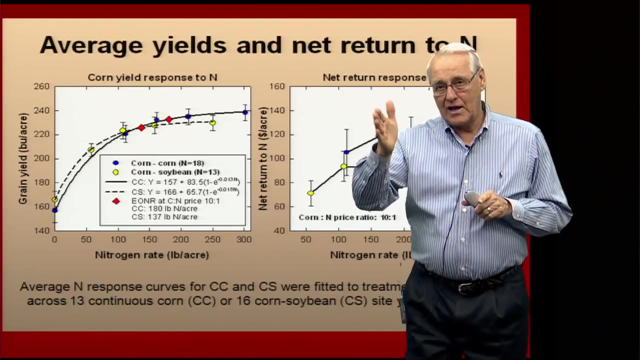 That's good news in two ways. Number one: if you aren't producing quite maximum yield but you're making maximum profit, that means you're making maximum money. If you remember the yield and the nitrogen, the nitrate curve, we know that at a point of maximum yield, 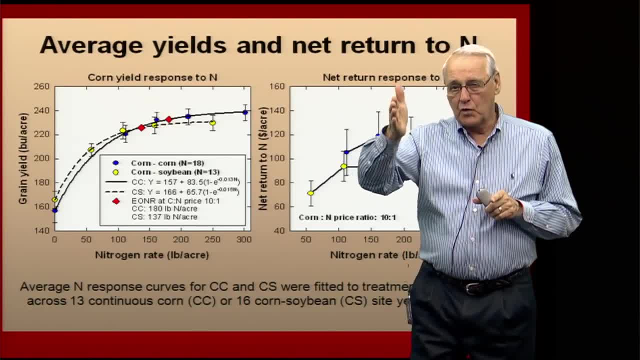 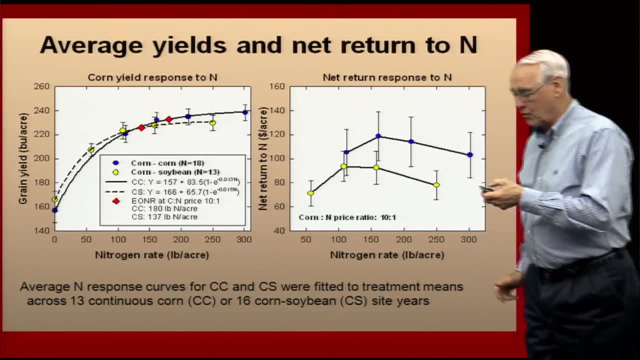 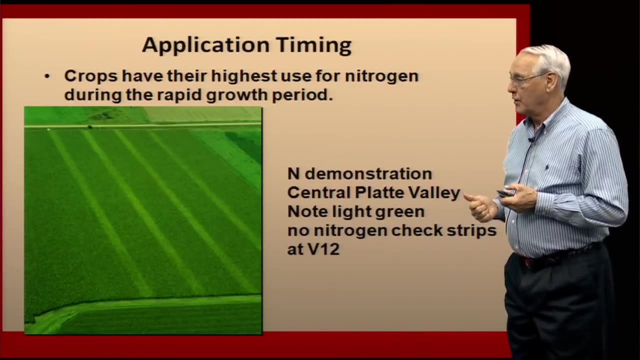 that's when we're really starting to increase our residual nitrate. If we're a little bit below that, we're going to probably have a soil that we don't have a lot of excess nitrogen left after we harvest the crop. Application timing of nitrogen is very important. 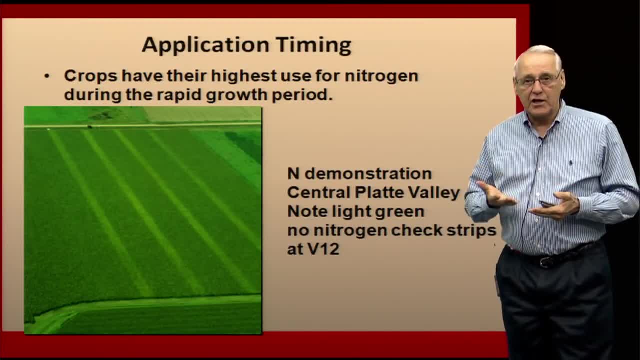 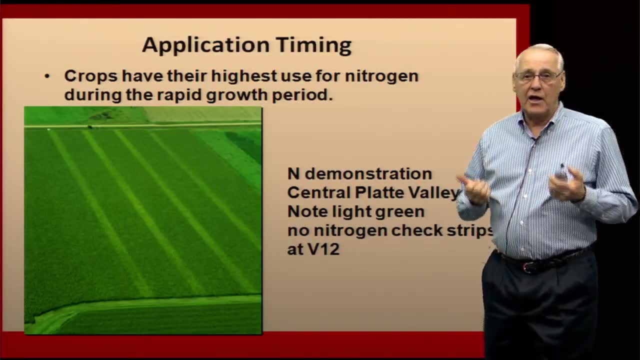 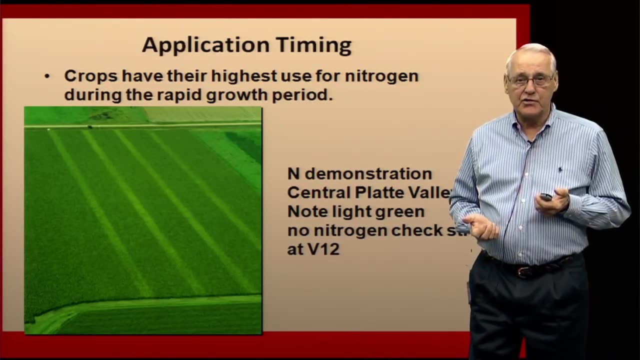 Earlier we discussed how the crop grows when it's taking up the nitrogen, how much of a root zone that you have the capacity to take up that nitrogen. We feel that delaying nitrogen application is one of our best methods of improving nitrogen use efficiency and reducing nitrogen leaching. 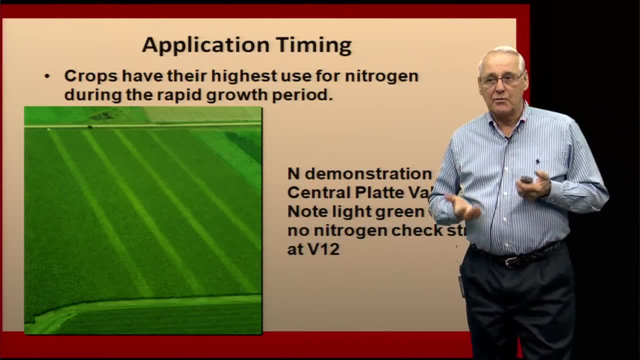 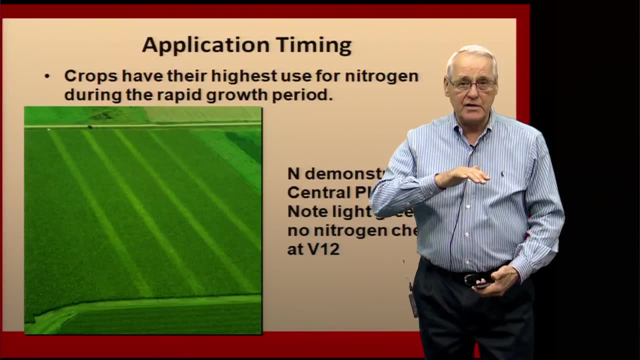 You need a little bit of nitrogen to get the crop started. But from the earlier discussion we know that that crop doesn't take up very much nitrogen until you get to the V8 to V10 stage. So if you can put a minimal amount of nitrogen, you're going to have a lot of nitrogen. 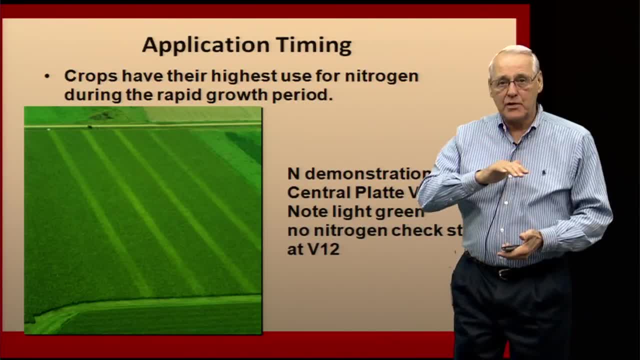 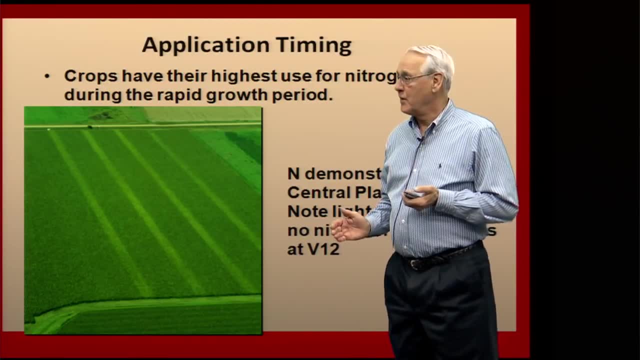 But if you can put a minimal amount on early, you also get by that period when we have our maximum leaching going on. And so over the years we've done hundreds of nitrogen demonstrations And some of the best ones that have been done. 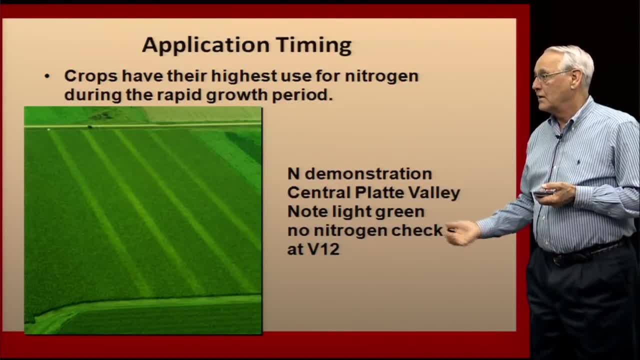 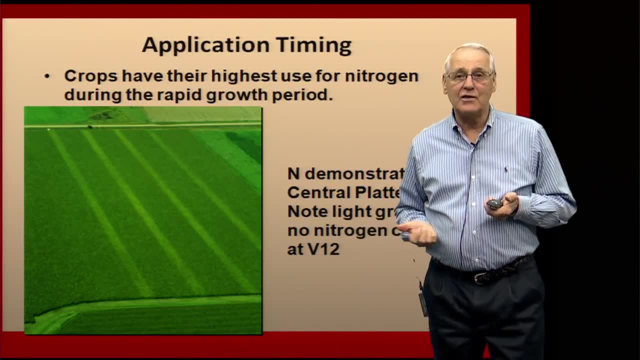 have been in the central Platte Valley where they've had a nitrate problem for years. We started talking about this when I was a young scientist back in the late 1970s. Back then we had areas in the central Platte. 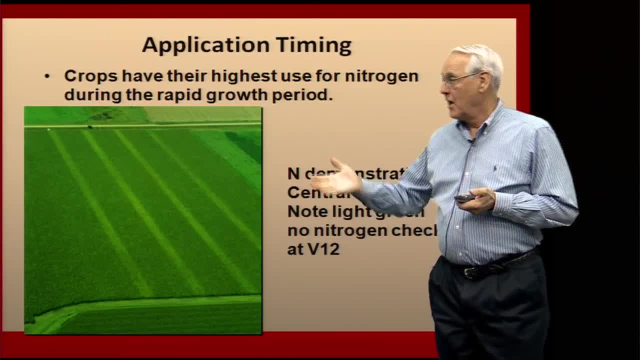 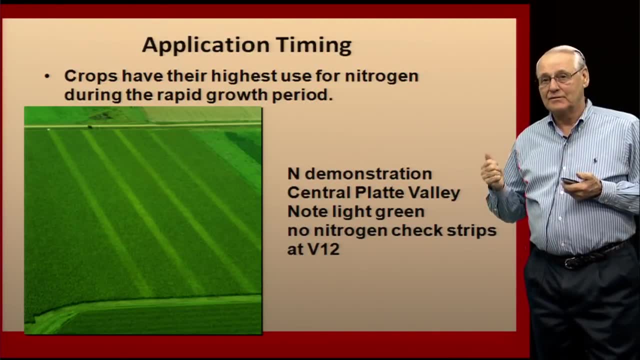 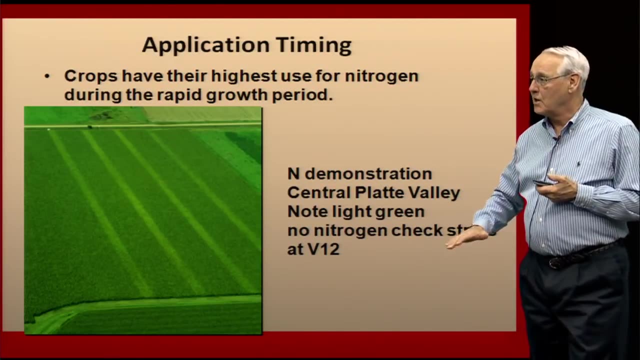 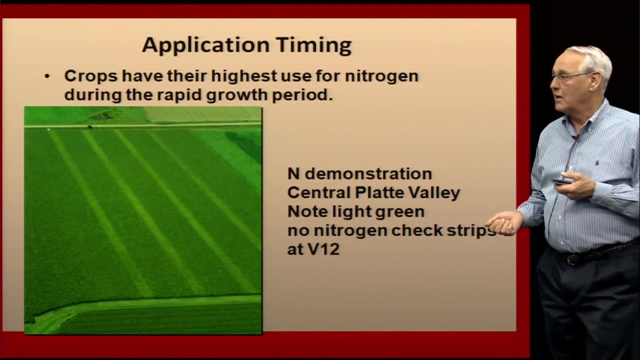 that had nitrate groundwater levels of 25% to 30%. After 30 years to 35 years of improved nitrogen and water management through the NRDs and farmer cooperation, that groundwater nitrate level has declined because of better nitrogen management And a lot of it was convincing farmers with these nitrogen demos. 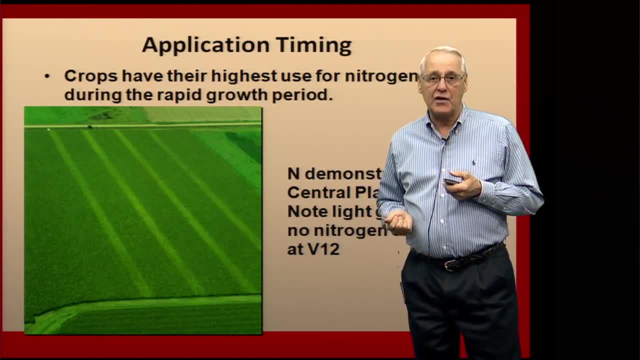 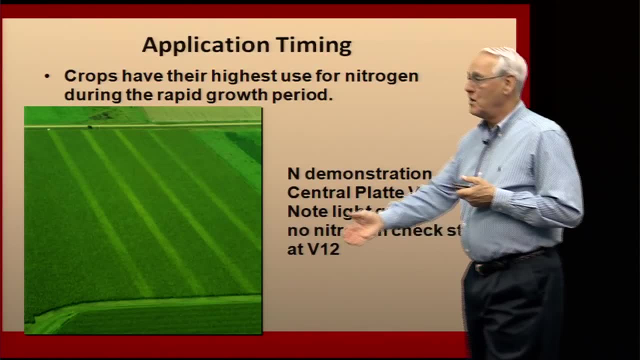 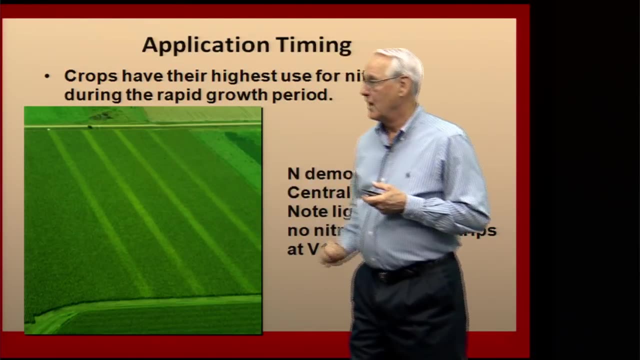 that were done to look at effective nitrogen rates for really getting the right nitrogen rate to get the right yield. In this plot you can see we have replicated strips. We had different nitrogen rates in here. We would always leave a check strip with no nitrogen. 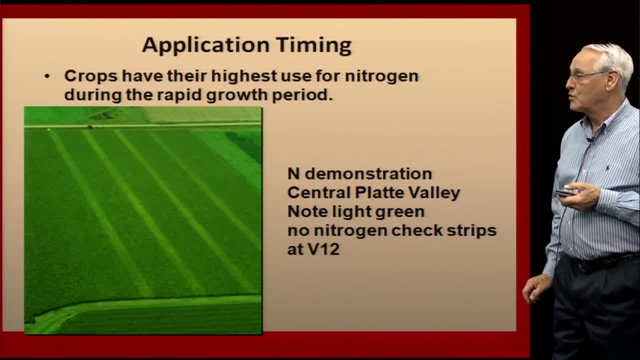 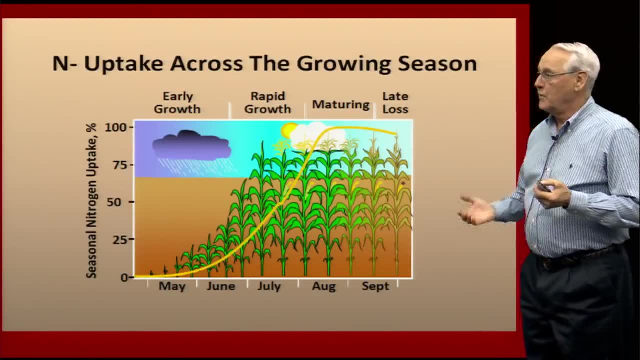 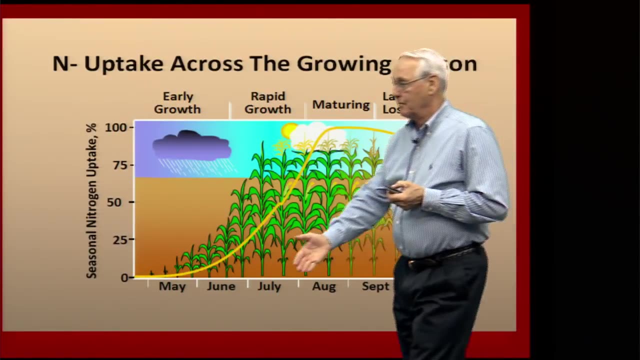 And that's very evident on those kind of yellow-green strips where those were. And this is about the V12 stage. So again, if we go back and if we look at nitrogen across the growing season in terms of the uptake early on, 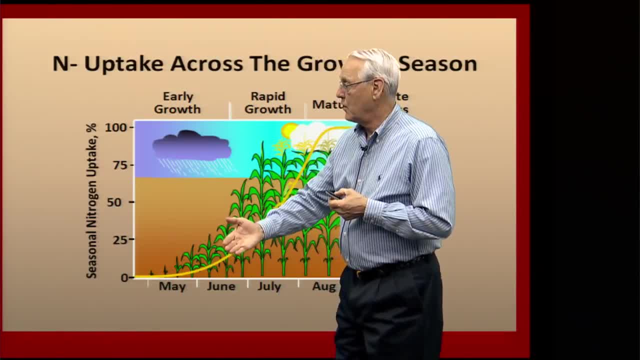 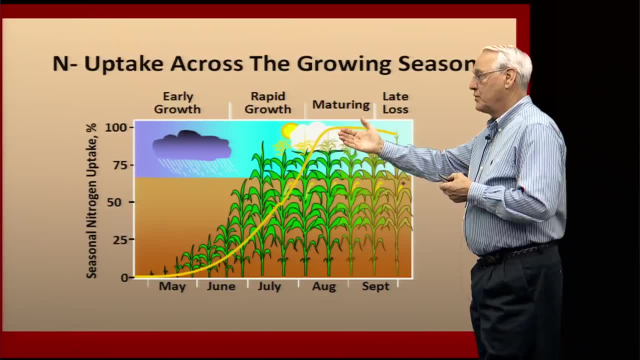 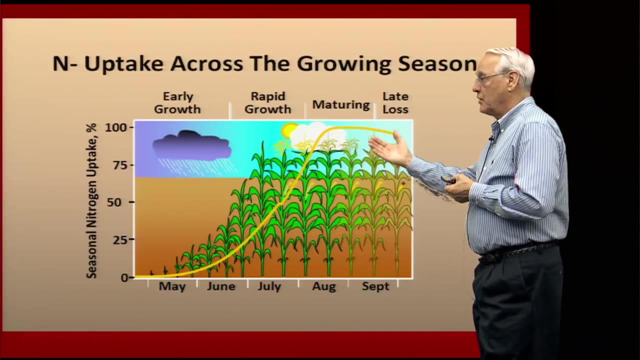 May and June: Not much uptake. It really starts to take off about the middle of June. We get a very rapid uptake which then reaches its maximum right at about tasseling time or early ear fill, And then that declines somewhat as we go. 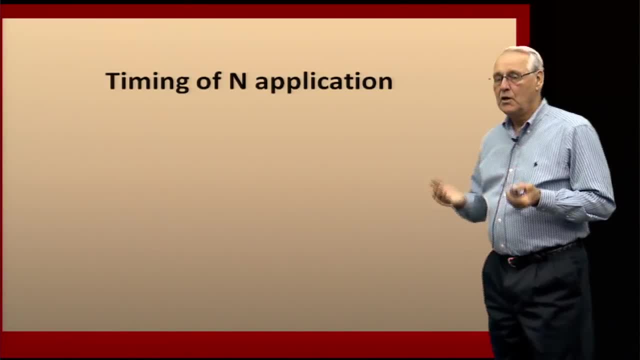 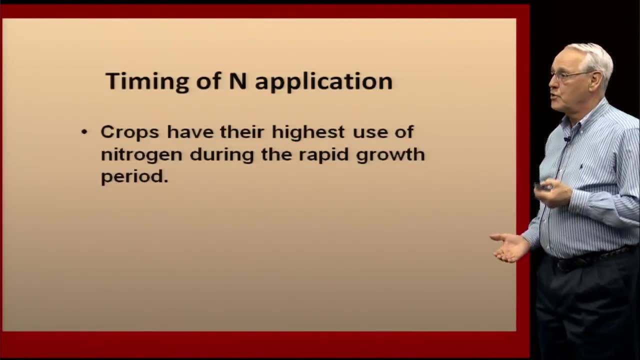 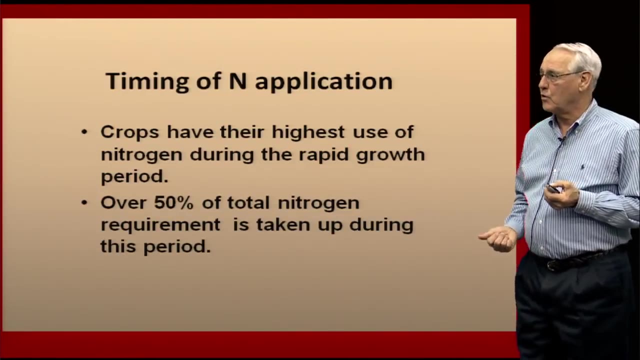 toward physiological maturity. All of this plays into the timing of the nitrogen application. Crops have their highest use of nitrogen during that rapid growth period. Over 50 percent of the total nitrogen that we take up in a corn crop is taken up during that period. 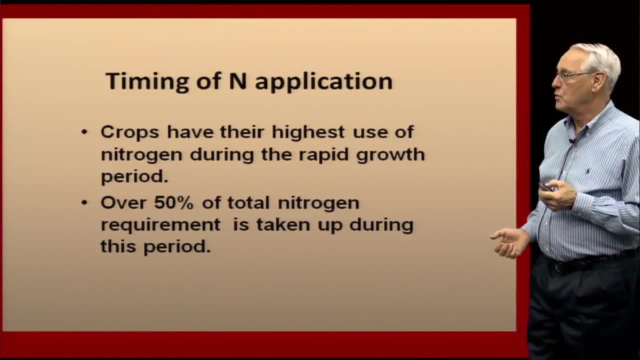 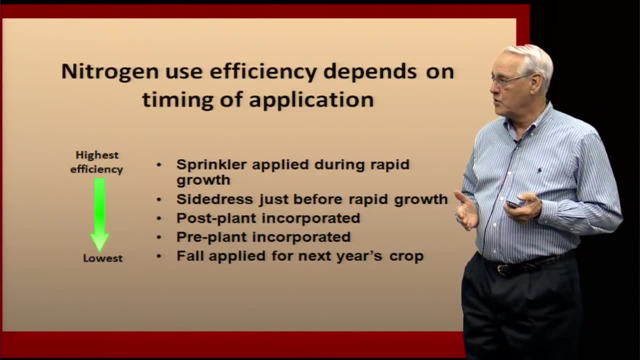 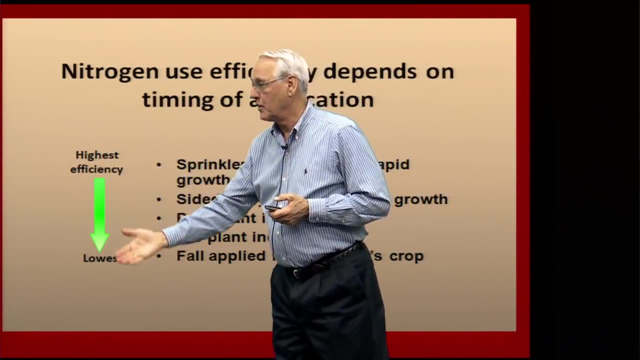 from about mid to late June to the middle of August, As we look at different strategies for nitrogen application, the ones that produce the highest efficiency. if we rank them from high efficiency to lowest, the most efficient that we can be is the C泡 content- Mansfield student. 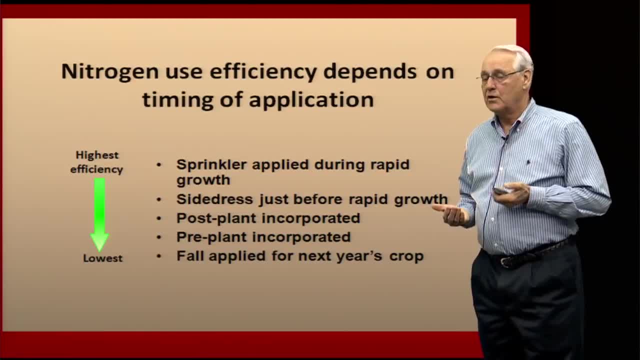 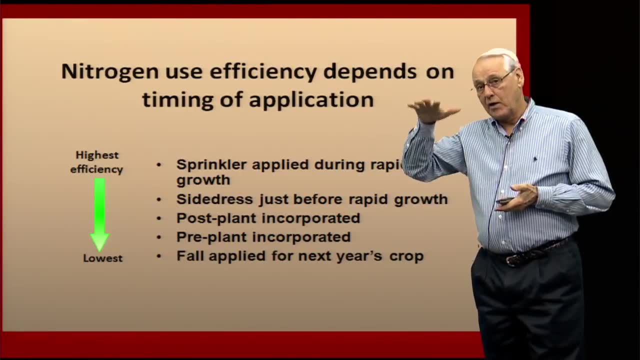 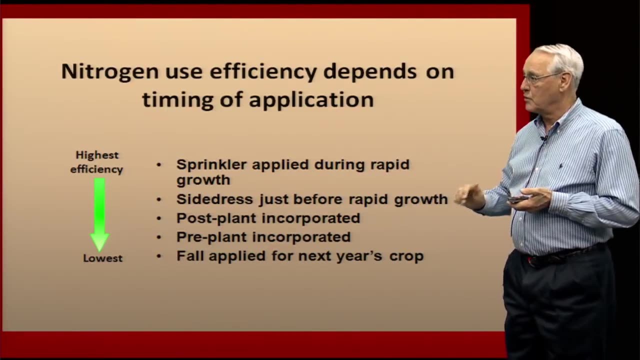 is sprinkler applying nitrogen during that rapid growth period. that's a time period when the plant is using maximum amount of water. our rainfall has decreased somewhat, we don't have the potential for leaching. that's when we can get the highest efficiency of our nitrogen. after that, a second best: 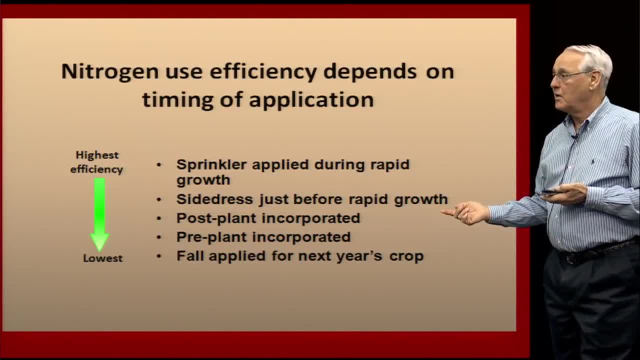 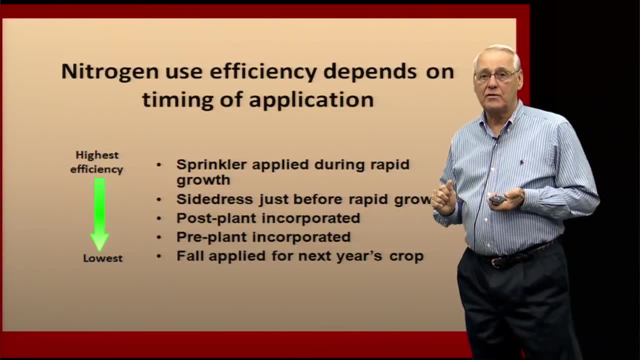 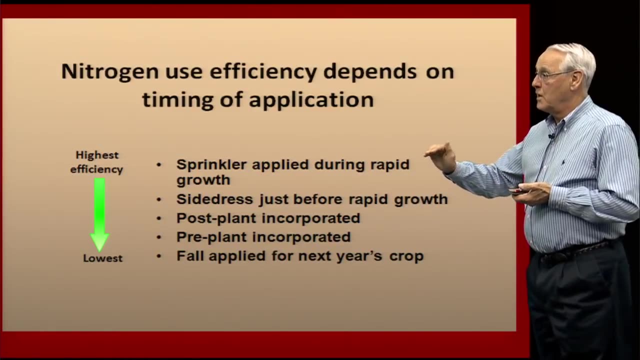 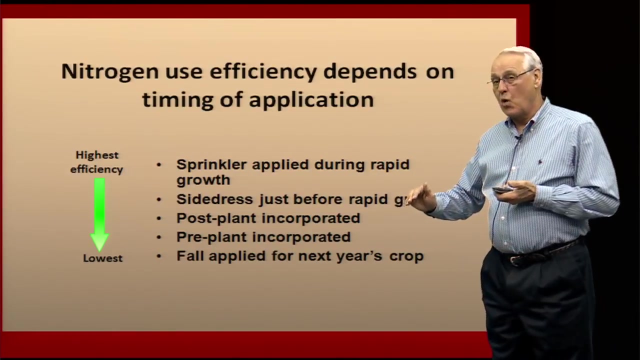 application or method would be side dressing at that v6 to v8 stage, putting on a small amount of nitrogen initially to get the plant going but then putting it on its side dress. in many cases- we have many years- we have equal efficiency between sprinkler applied and side dress. the next option that isn't quite as good. 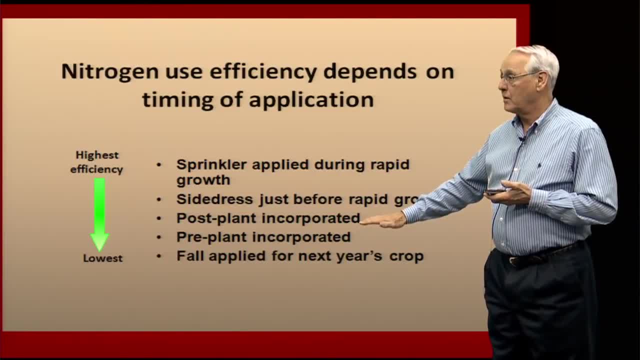 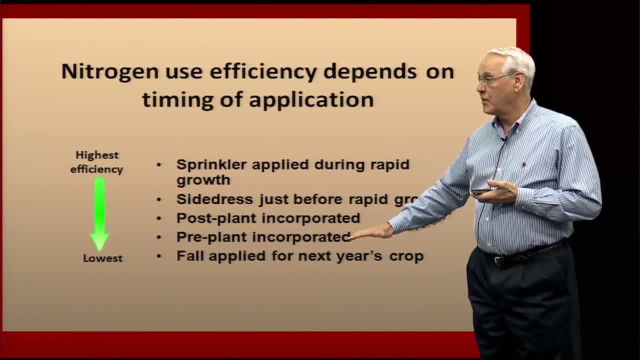 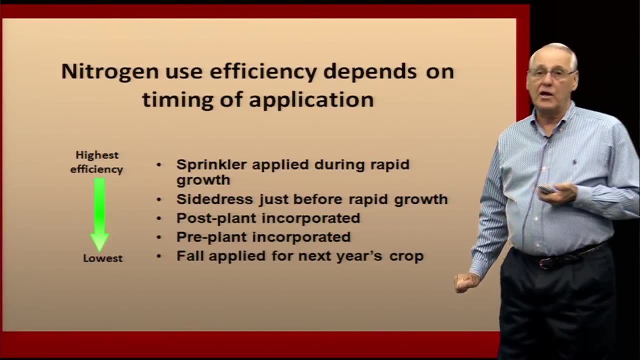 is waiting and putting that nitrogen on post plant. the next, that's one that we will lose nitrogen a number of years. in eastern nebraska is a pre plant incorporated and really our worst option in terms of nitrogen use efficiency is fall applied for the next year's crops. we do have nitrification inhibitors. we have worked. 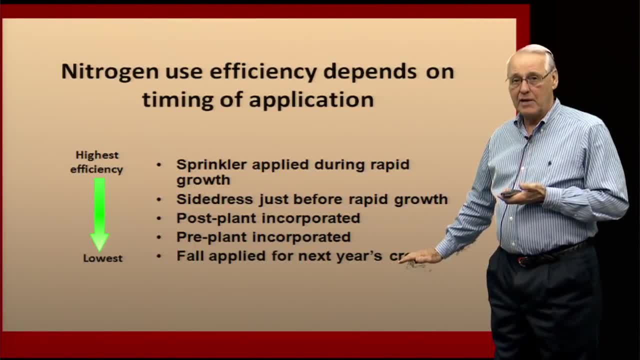 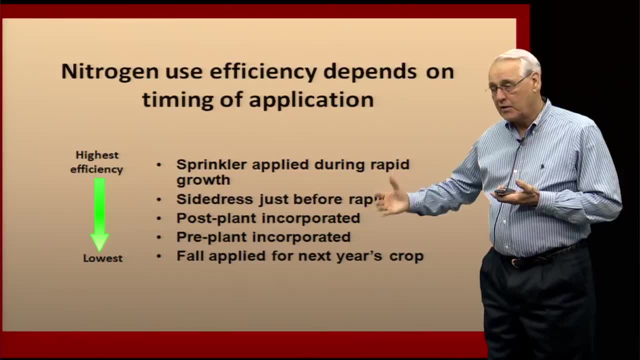 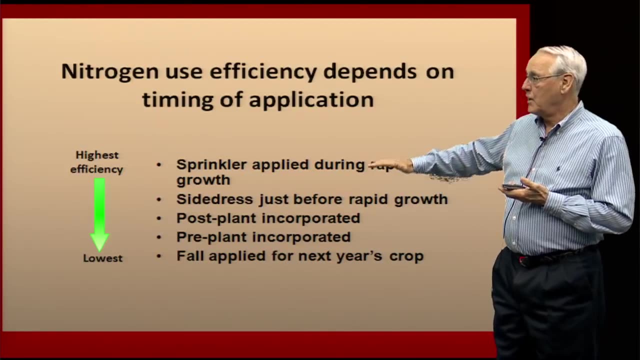 with nitrification inhibitors. with fall applied anhydrous ammonia that performs very much like pre-plant incorporated. it slows the nitrification but really in effect it's not much different than pre-plant applied nitrogen. so if we're thinking about nitrogen use efficiency, we're needing to think about 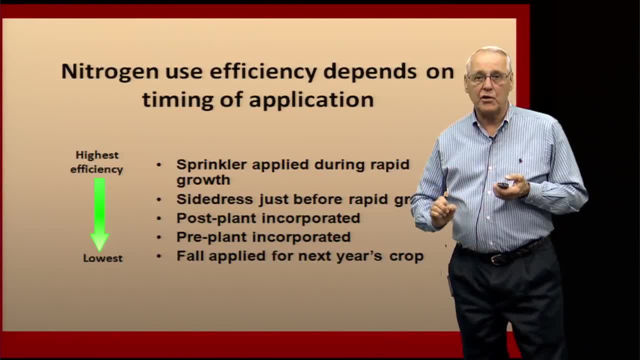 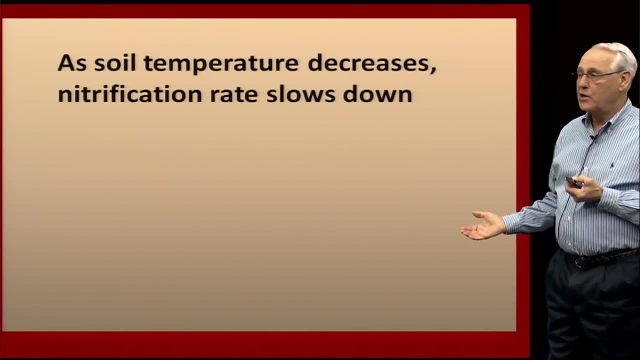 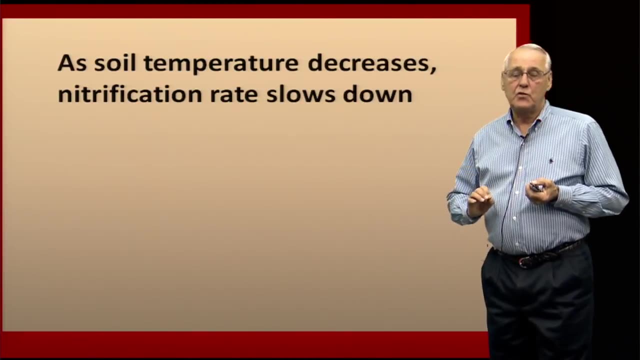 nitrification starts, so it hasn't been a massive change in tailings and or growth shoes. what we're looking at is now a might be mycogen harus engine and cabbage ku toppings is very hoje restroom. most of 9 ministries, the chile branch dry. 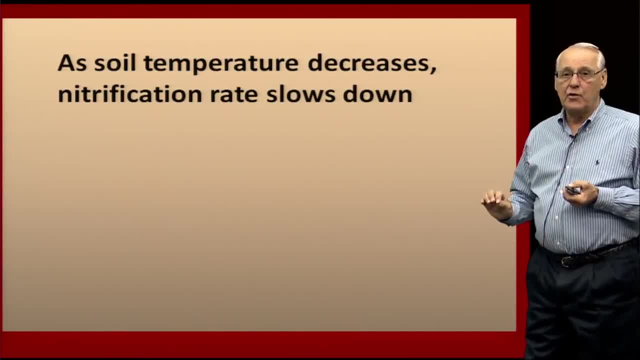 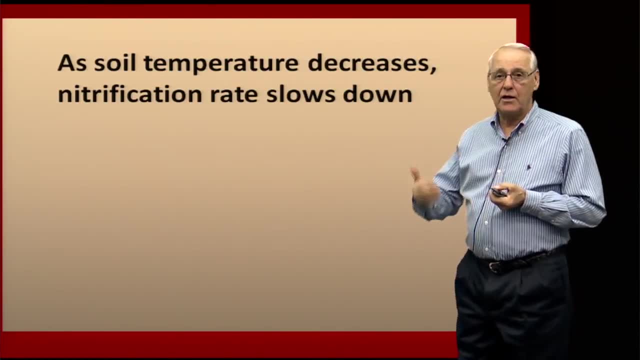 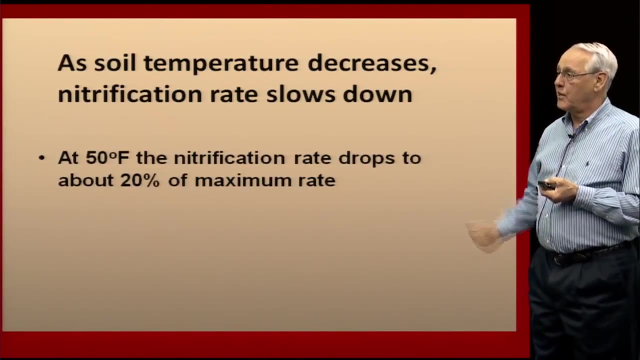 we've got a shallower propertyHave a navement год contract and we'll continue to put in chatting. you can see, simply you can see- is affected by soil temperature, because that affects the bacteria that do that conversion. At 50 degrees Fahrenheit the nitrification rate drops to about 20% of. 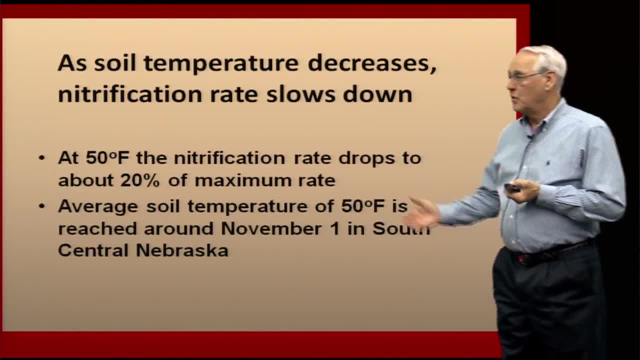 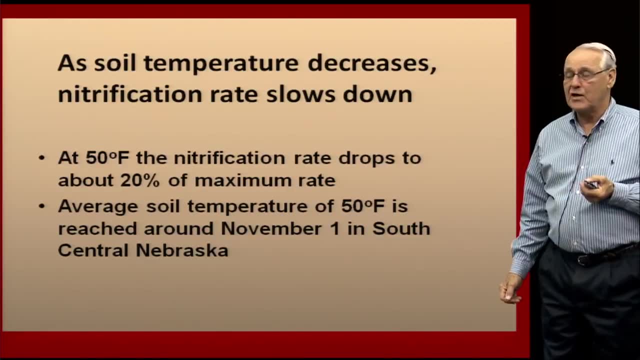 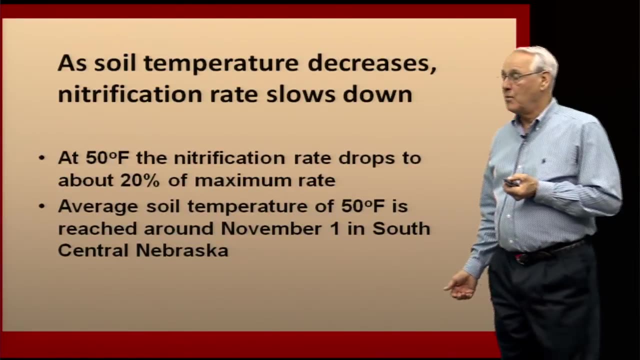 its maximum rate. So if you are going to fall apply, we tell farmers they should wait until the soil temperature is below 50, and that usually happens about November 1 in south central Nebraska. Also, the other thing with fall application: if that really is a preferred method, it probably is a good. 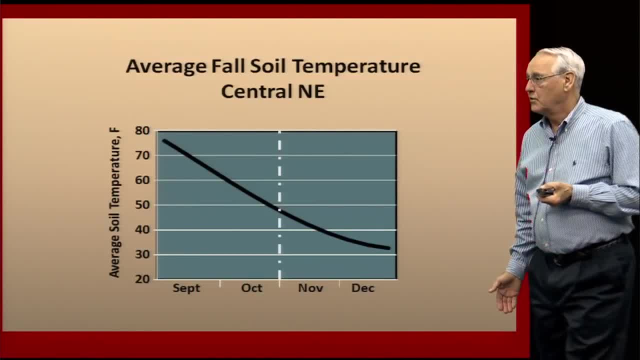 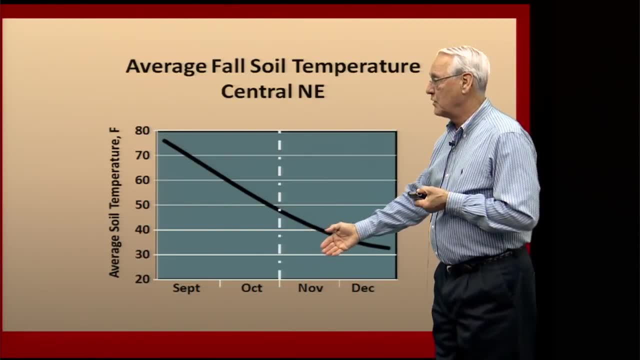 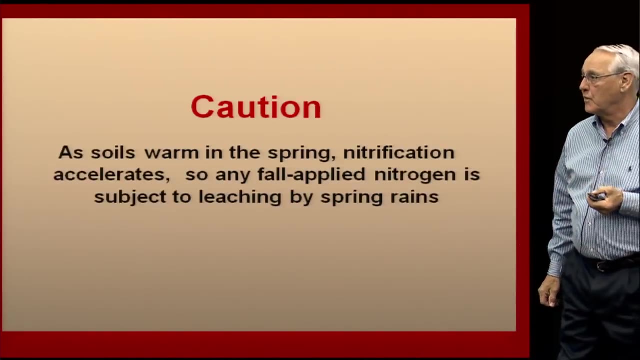 idea to consider using a nitrification inhibitor. So this is just a change in the soil temperature from the first part of September through November into December. You can see we hit that 50 degree threshold somewhere about the 1st of November. The thing is that in the springtime, when soils begin to warm, that 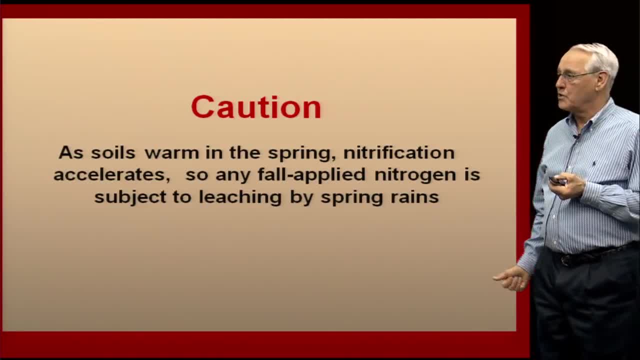 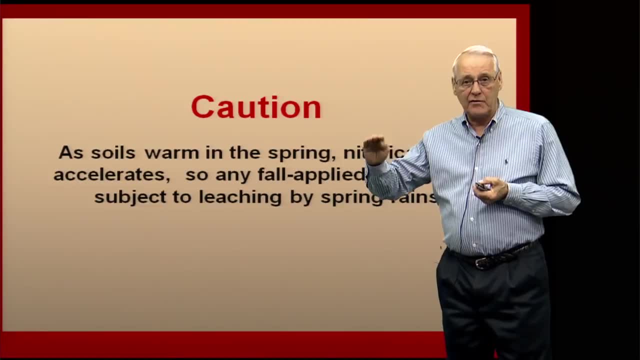 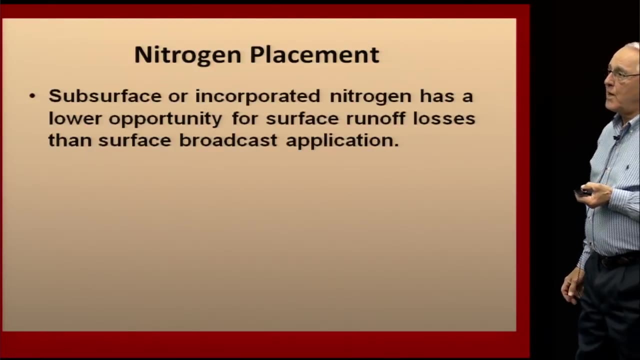 nitrification accelerates so it shows that the soil temperature is there. So any fall applied nitrogen that converts to nitrate can be subject to leaching by those spring rains during that high rainfall period of those month- May, June, early part of July- When we 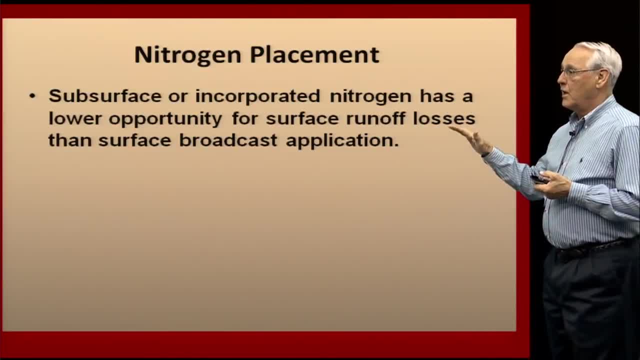 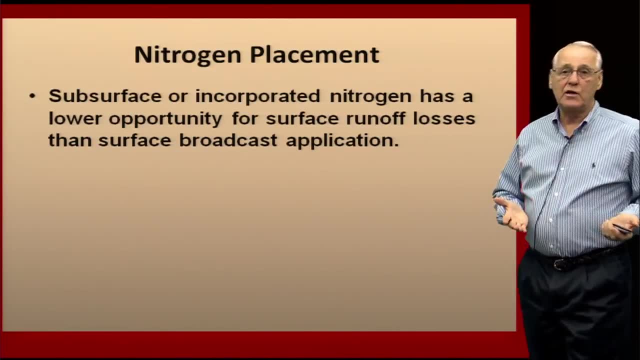 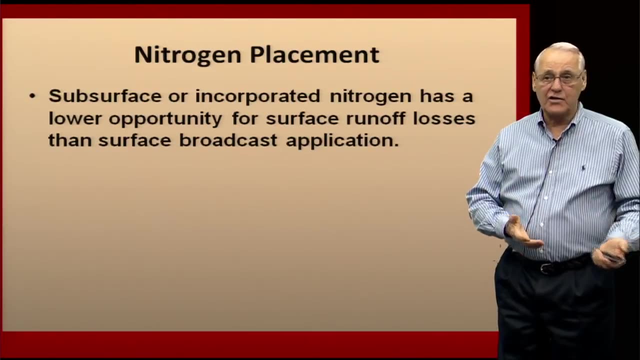 think about nitrogen placement and other losses of nitrogen. subsurface or incorporated nitrogen has a lower opportunity for surface runoff losses than surface broadcast application and we have a nice gentle half inch rain. we're probably not going to lose anything in surface runoff If we broadcast either dry or liquid fertilizer nitrogen if we have. 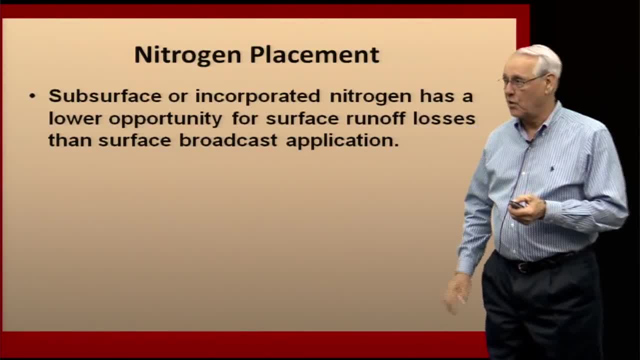 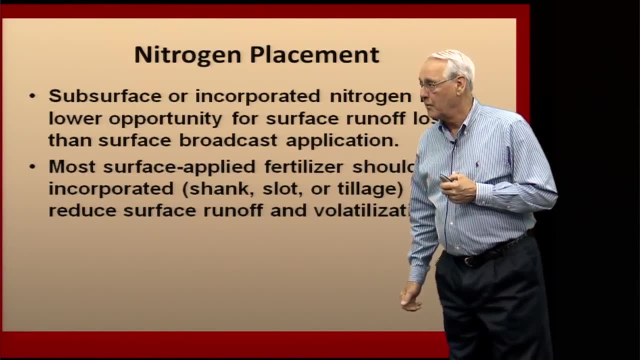 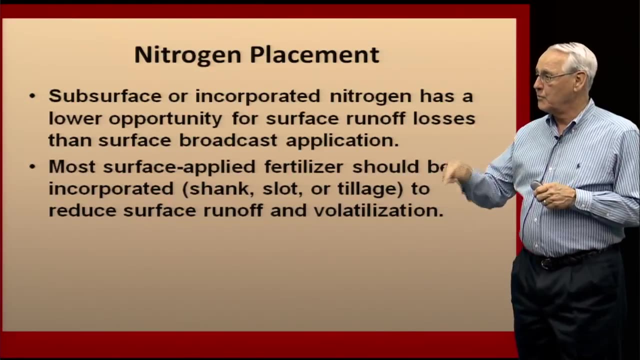 a big two inch rain, we are going to lose some in surface runoff and that's why subsurface or incorporated nitrogen is generally a good safeguard to not lose it. that way, Most surface applied nitrogen should be incorporated. That can be done with a shank, a slot, some form. 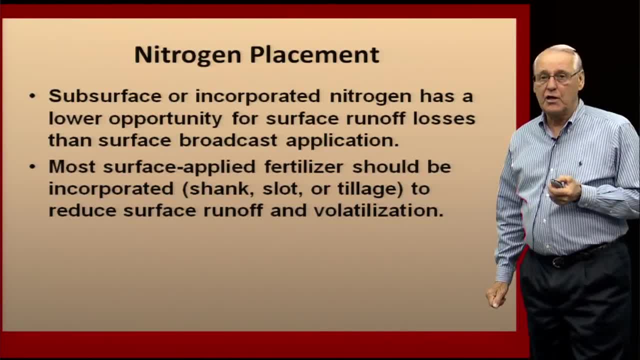 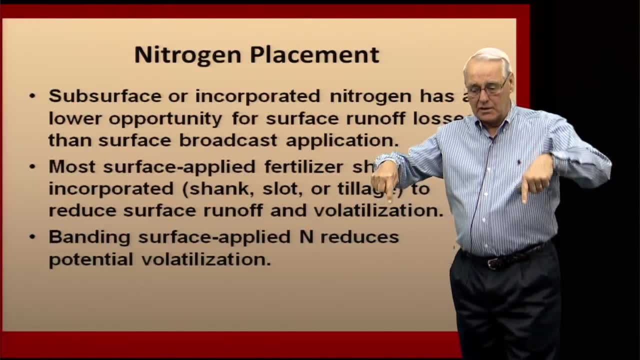 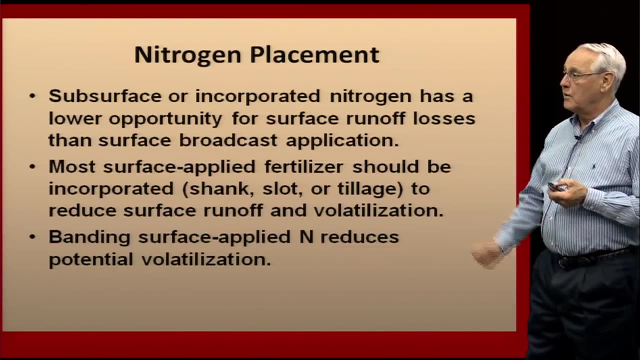 of tillage to reduce surface losses and also to reduce nitrogen volatilization. Surface banding of nitrogen, where we're basically dribbling it on every 18 to 24 inches, reduces potential volatilization. The other tools that we have these days we do have a number. 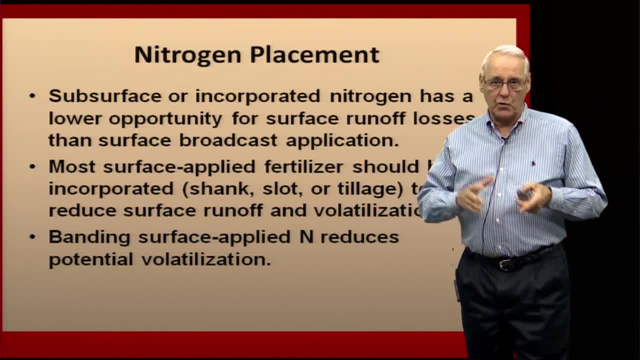 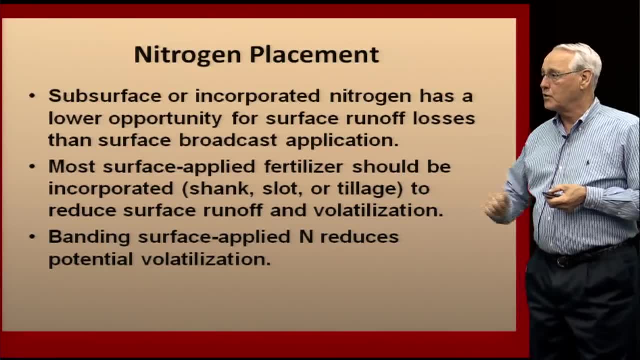 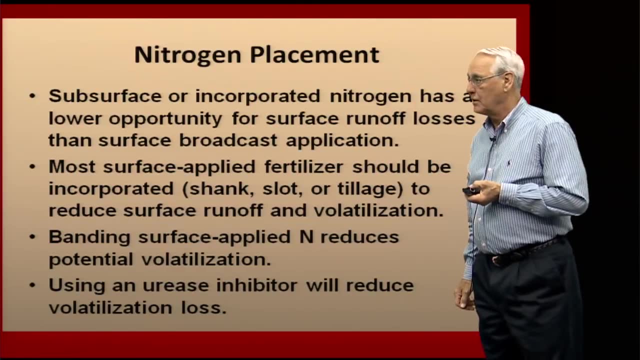 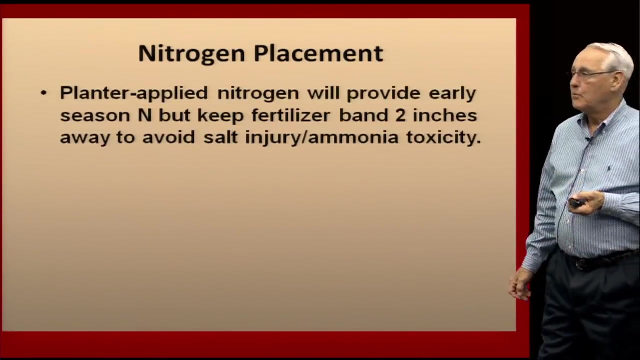 of urease inhibitors which slow the conversion of the urea portion of fertilizers, whether it's dry or whether it's in liquid. It slows down that conversion and can help reduce volatilization. in high pH or high situations where we would volatilize, that nitrogen And that urease inhibitor will reduce volatilization. 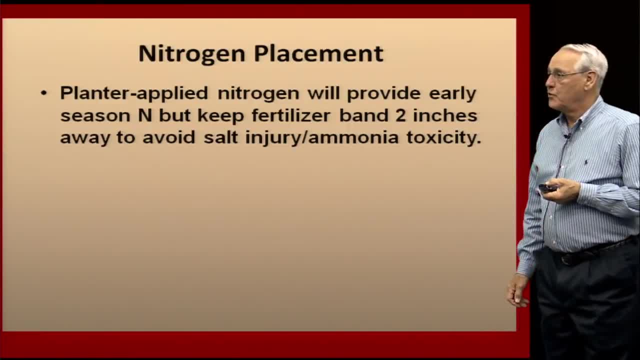 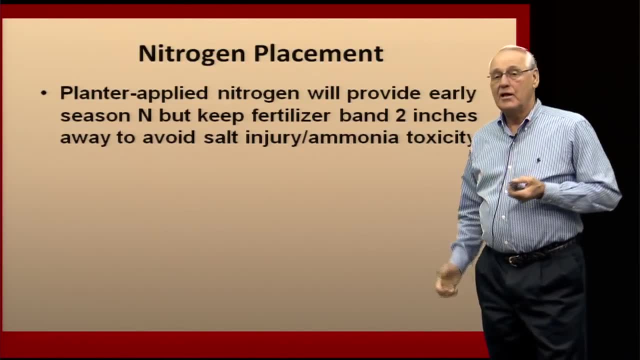 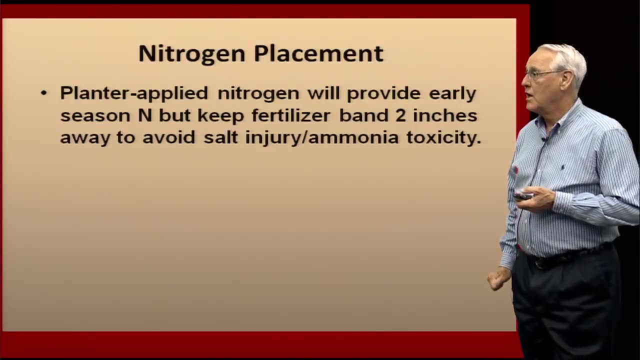 Planter applied nitrogen will provide an early season shot of nitrogen. A lot of farmers use 20 to 30 pounds of nitrogen in a starter band. That's more than enough nitrogen to get that crop up to that. If you do that, though, you need to make sure that that fertilizer band is at least two. 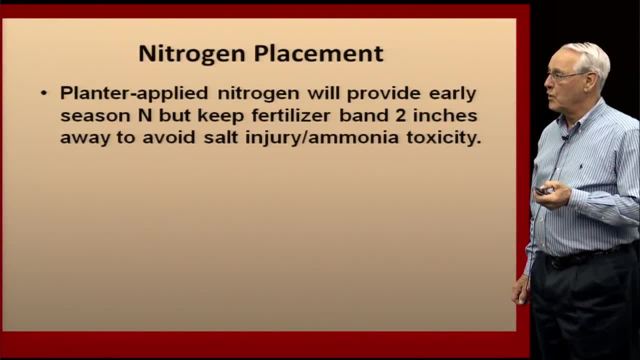 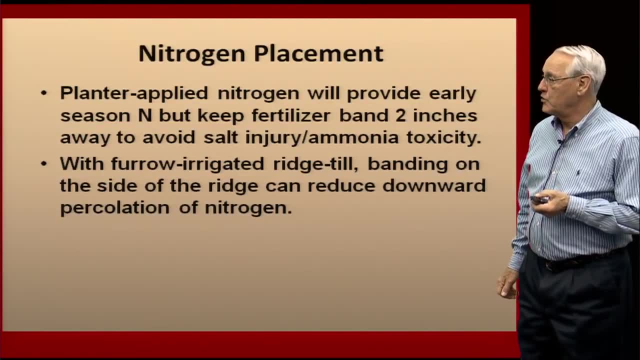 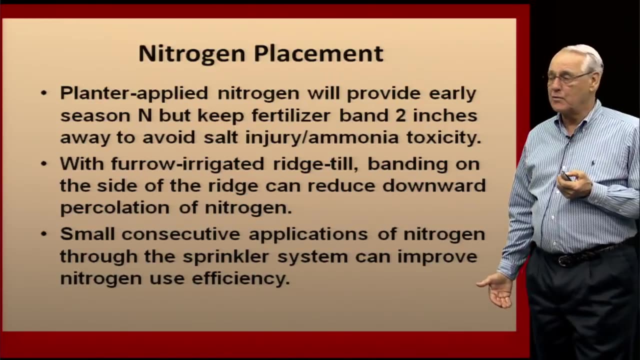 inches away from the seedling to avoid salt injury or ammonia toxicity. With furrow irrigated ridge till banding on the side of the ridge can reduce downward percolation of nitrogen, But we feel our most effective and efficient means of applying nitrogen is split applying. 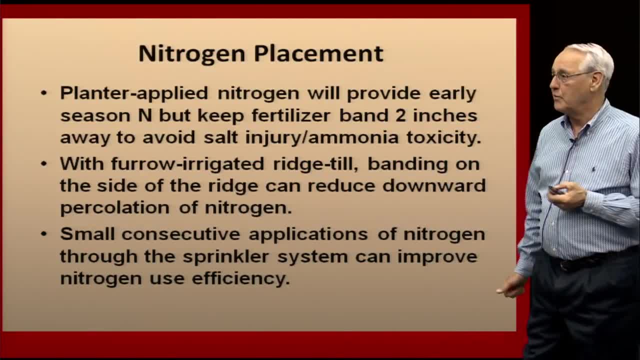 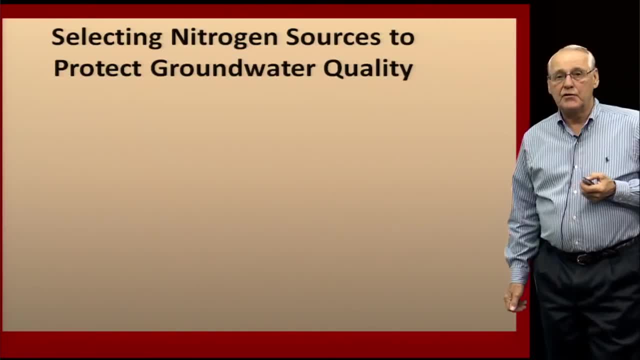 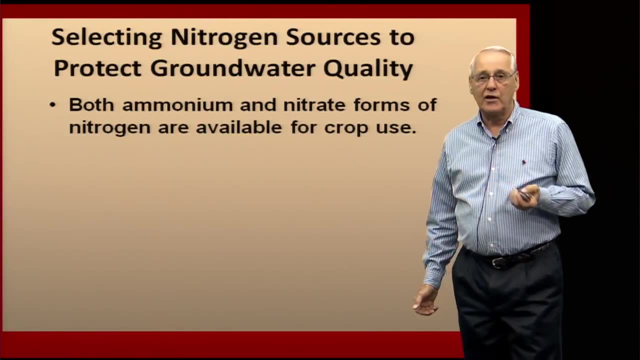 nitrogen is split into two times as we put water on during the growing season. If you have a center pivot and that can really improve the nitrogen use efficiency. Different nitrogen sources for protecting groundwater quality, Both ammonium and nitrate forms of nitrogen, are available for the crop. However, the crop does take up probably 80. 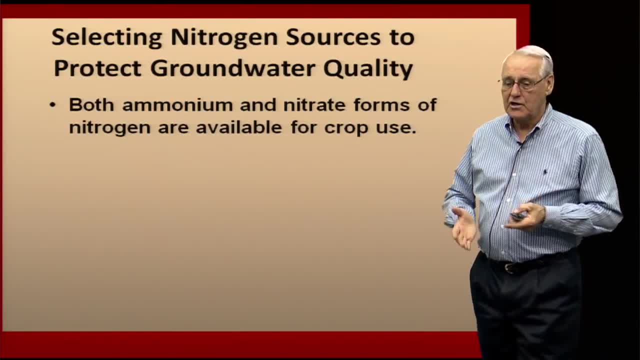 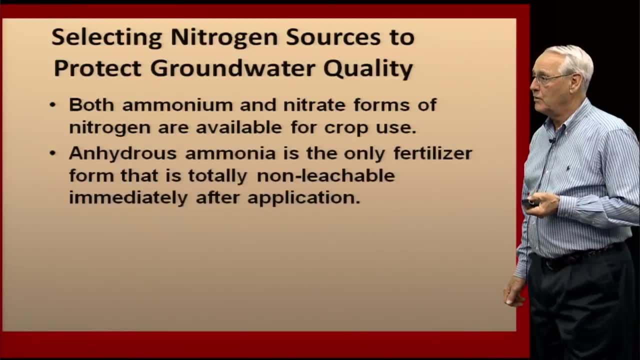 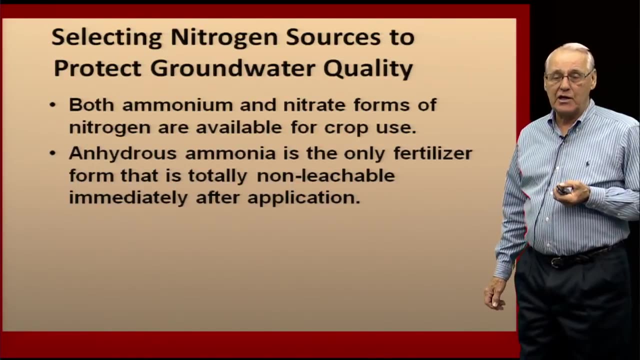 to 90 percent of its nitrogen as nitrate nitrogen. So ammonium forms need to be converted to nitrate And that happens naturally by the soil bacteria. Anhydrous ammonia is the only fertilizer form that is totally non-leachable. immediately after application, You can put on ammonia, have a four-inch rain, you can. 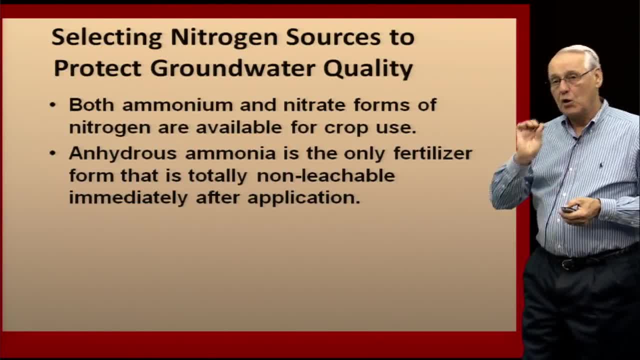 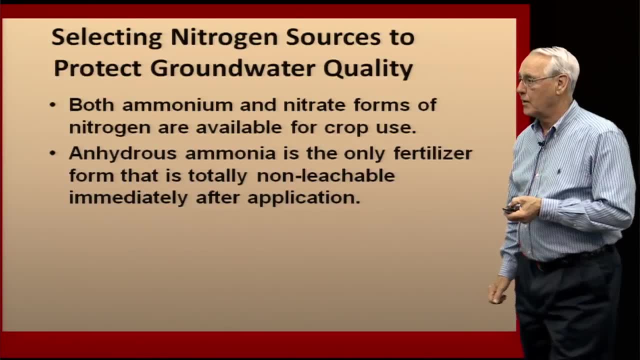 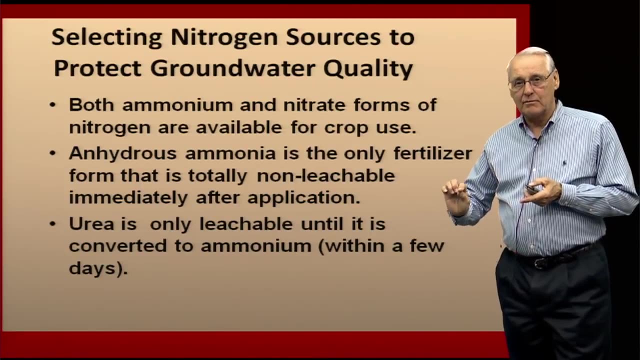 move water. the ammonia is held tightly to the soil. it won't move Once it nitrifies, though, nitrate is the soluble form of nitrogen and it moves with the wetting front of the water, Urea, before it is converted to the ammonium form by the enzyme urease. that's 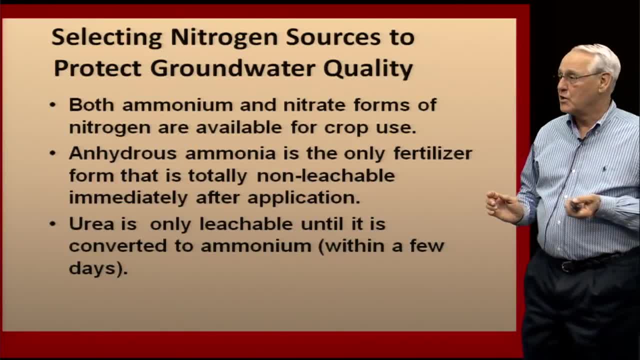 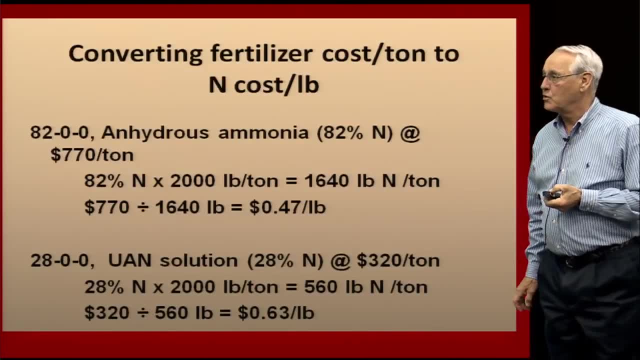 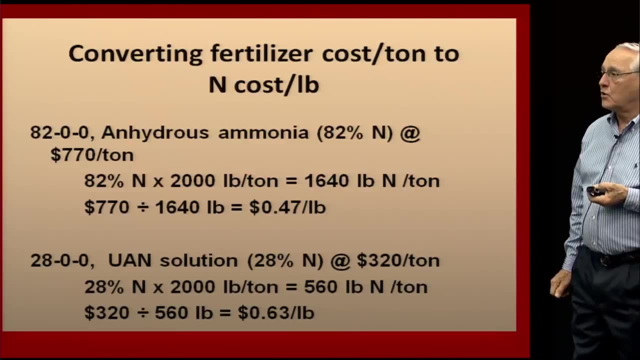 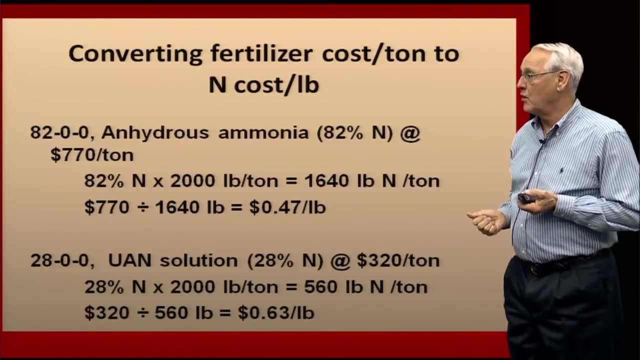 in the soil actually can be leached. But that conversion to ammonium happens fairly quickly, probably within one to three days of application. Just a little bit of fertilizer arithmetic and looking at the cost of nitrogen This winter. anhydrous ammonia earlier was running about $770 a ton. If we calculate that out, it turns: out to be about 47 cents a pound of nitrogen. Most of our dry and our liquid forms of nitrogen, because of increased manufacturing costs, do cost more. Nitrogen solution is 320 a ton versus 770.. But when we calculate it out on the cost per pound of nitrogen at that price, 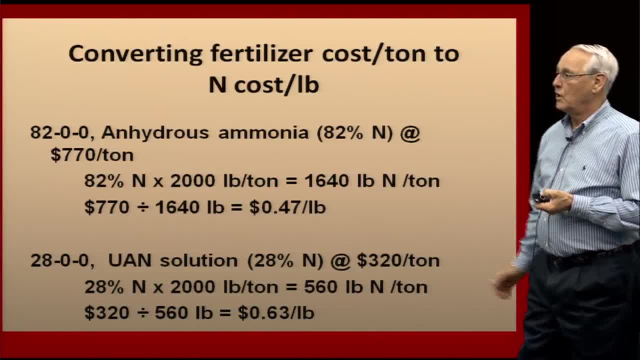 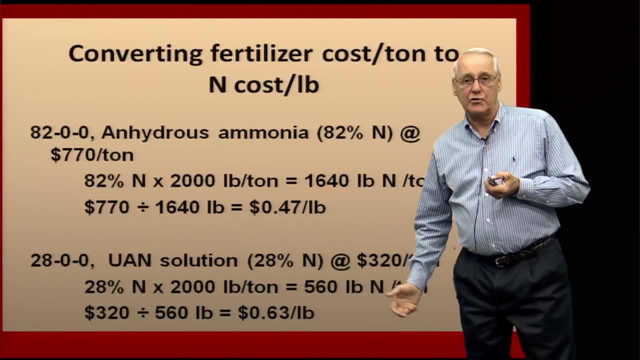 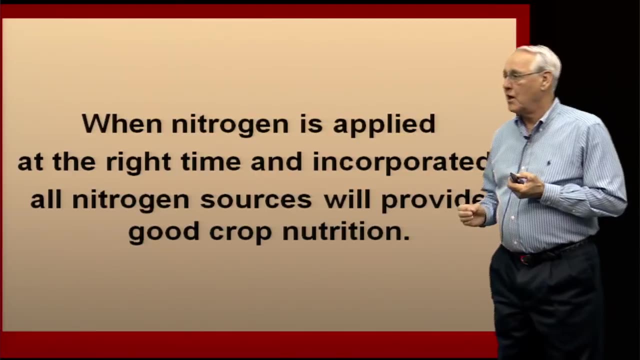 it would be about 63 cents per pound. Currently, uh, ammonia's running around 50 cents a pound or more, and dry and liquid forms of nitrogen are running about 60 cents per pound of nitrogen. The thing that we know when we apply nitrogen at the right time and add to it��도 and split. 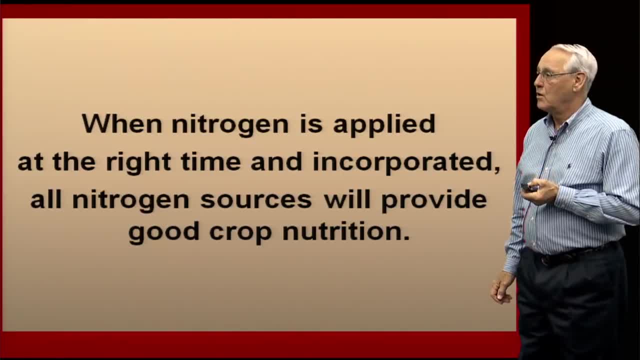 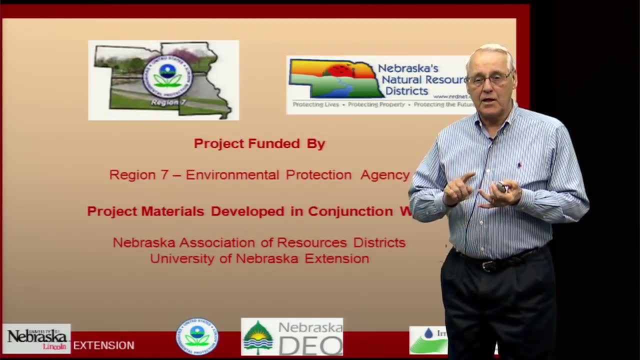 it as a part of that right timing. all nitrogen sources will provide good crop nutrition and good nitrogen management, coupled with good water management, will provide a very good resources as well. The focus is also to grow production For hedge gas. uh, as it's crucial we have to.